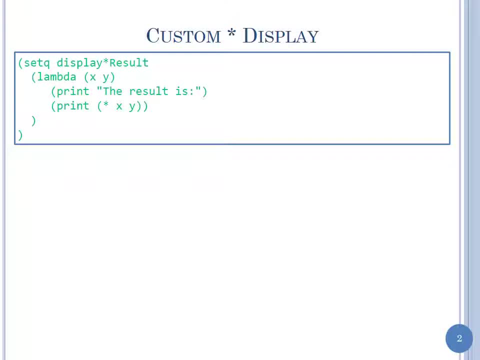 already set Q and lambda to go and write this particular thing And I can then say: fun, call display. Again, if you're getting put off by display star result because you don't see that in Java, that is valid, you can have. 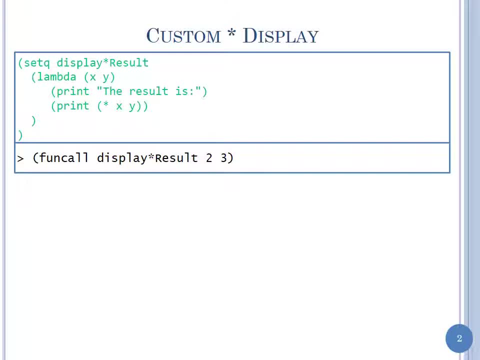 anything be a function name that doesn't have spaces. Okay, so I do fun. call display, result two, three, and, and I'll get. the result is six. Okay So, and like I said, I'm doing some custom. That's just a function. So far, so good, Okay. 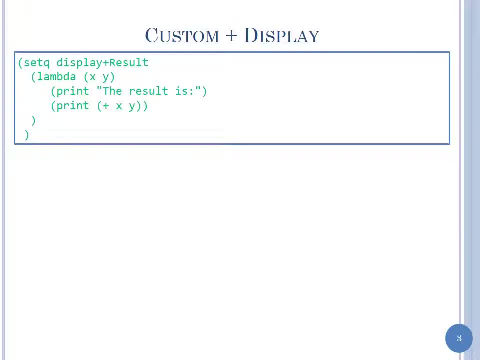 And I might later go and custom plus display also And I can say: fun call display plus result I can get the result is five. The result is five. is what, what, what, what? the function printed out and interpretive prints out the extra five arguments. So why did I go? and 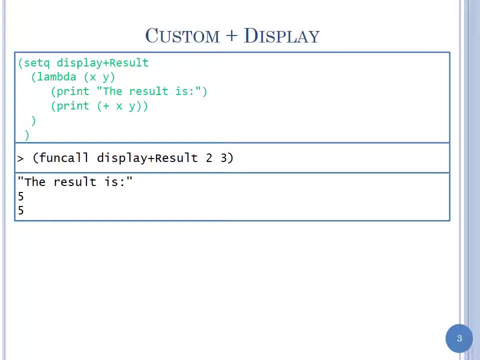 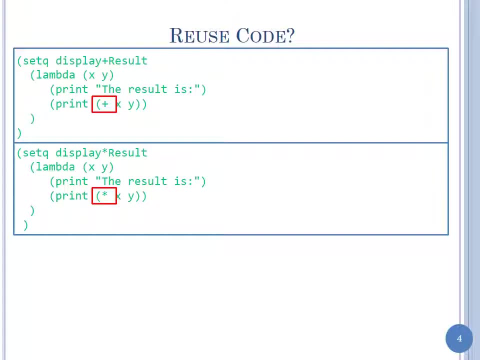 put these two functions. they're pretty simple functions, nothing you do to learn from them, But that you know. now I want to get into, put my reusability hat on. I've got two functions: display star and display Plus. okay, I copied and pasted the code from one to the other. 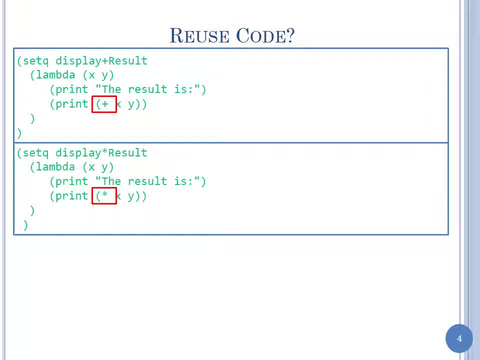 to create the other code, And the difference really is in the way the functions are named, of course, But the only real difference is that in one case I'm calling plus and the other place. So could I create a single function? Could I? Could I do that, Could I do that? 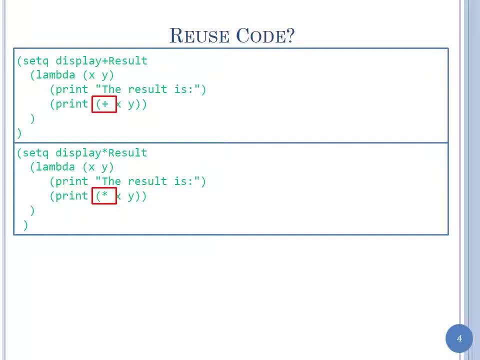 Yes, Okay, How could I do reuse, Could I? How could I remove the reuse, Remove the duplication here, and yet achieve the result of having a custom display of the star result and a custom display of the plus? So I guess that 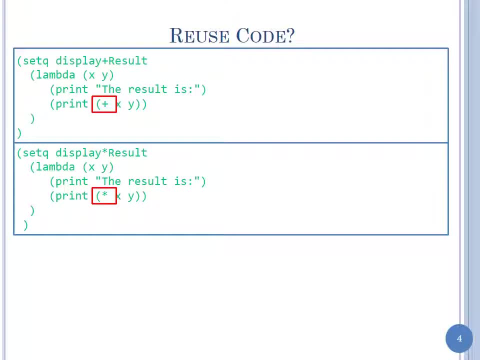 You can store the result somewhere and then. and then do what? then print the result. okay, You guys get that. So, but then for every pair of arguments I have to go and store the result right? So I do want the flexibility to go in: sum up anything and multiply anything and display. 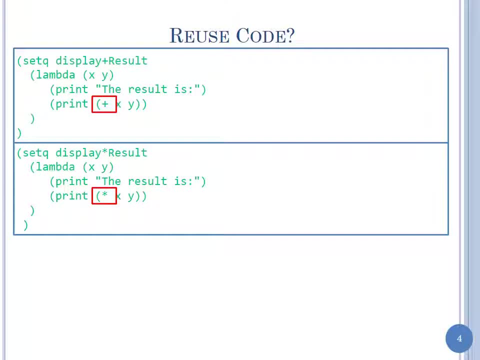 it properly. So what's the difference here? yeah, so that's what I'm hinting here, right, That somehow the plus and star should be an argument, should be a parameter to a function rather than hardcoded. You think of generics. what do? what do generics? do they make types as parameters, so that 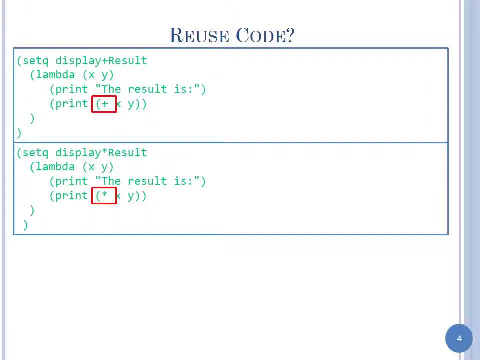 we don't have to go and create- And here I'm saying: let's go and create functions as parameters. okay, So that's now. you see, so far, what we've done with Lisp is: yeah, we've done recursive programming, but recursive programming is something that you could easily have done in Pascal. sorry, 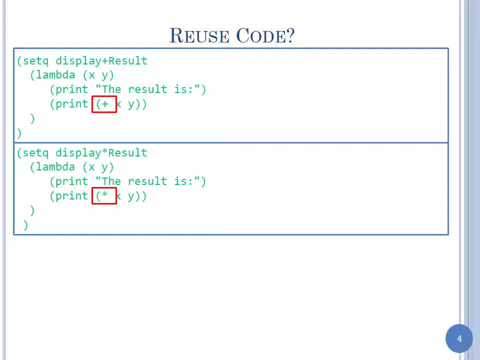 that was my first language- Java or other languages- And now we're getting interesting, which is also something that is not too alien to programming in C or Java, So I'll make- I'll have a display result that takes not only the x and y as parameters. 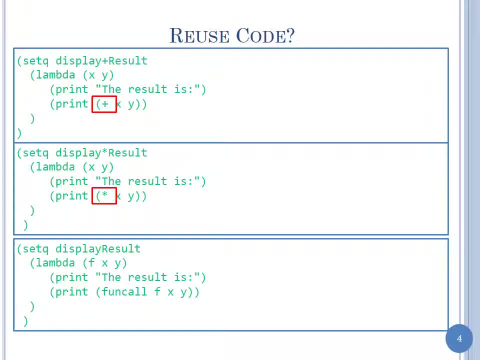 but also a function as a parameter. okay, Functions are values that can be passed as parameters, and where I was doing plus xy, I'm going to do funcol fxy. Now we have fun. you know this is- this is sort of fun arts. okay, functional arguments. 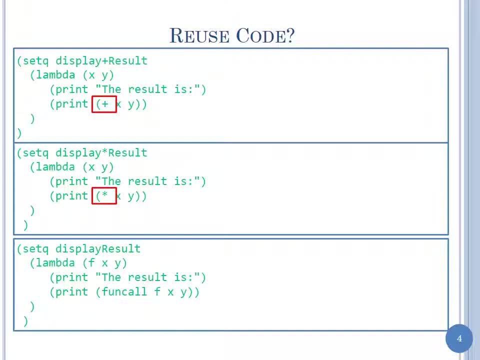 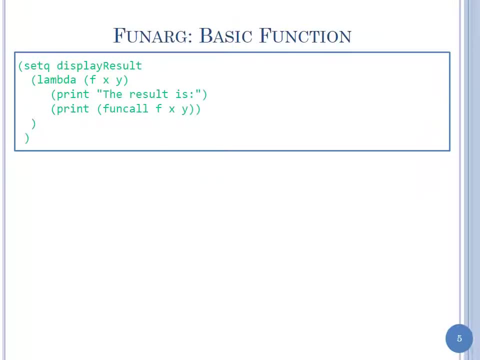 Questions. I can. now I have this function display result, which takes f as this argument, and I can go and say: funcol, display result plus two, three, Okay, Okay, Okay, Put on your tracing hat: 3 Funcol plus two, three. 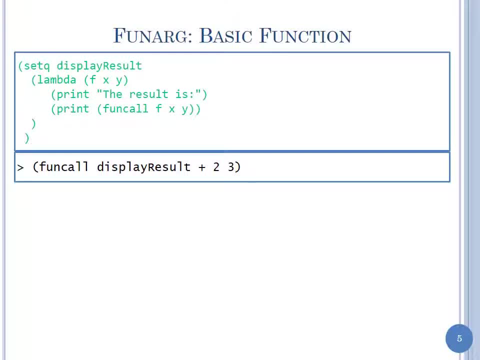 Funcol is going to do what? Evaluate plus 2? So what? what should the first argument of Funcol? evaluate? to Evaluate, to Evaluate. to Who is that Very good, Please go and put that. That's excellent answer. Yes, lambda expression. 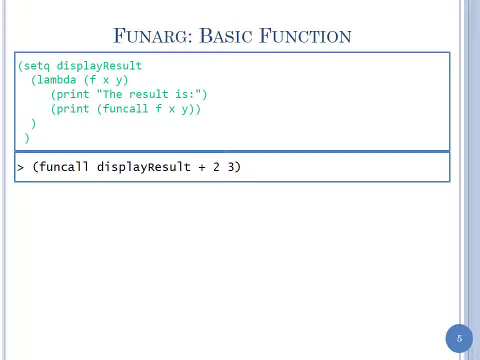 Is plus bound to a lambda expression. Plus is a basic function Plus EQ atom. these are not lambda, Okay, So you get some garbage message. Okay, the list gets totally confused. Okay, but we are there. So what should I do now? 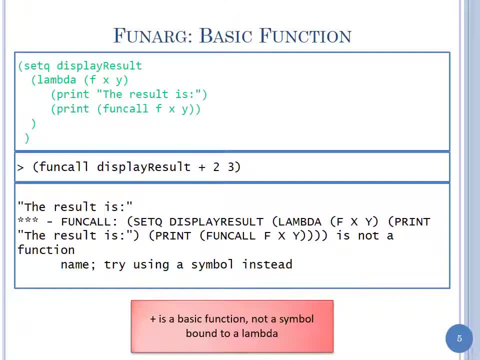 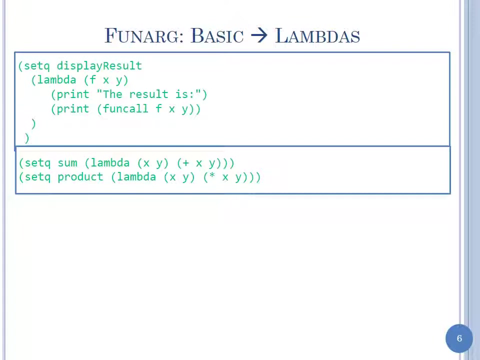 So plus is a basic function, not a symbol bound to a lambda. Okay, this is important Questions. Okay, So I can then say: okay, you know, we'll just define sum. We'll define a sum and a product as a lambda expression. 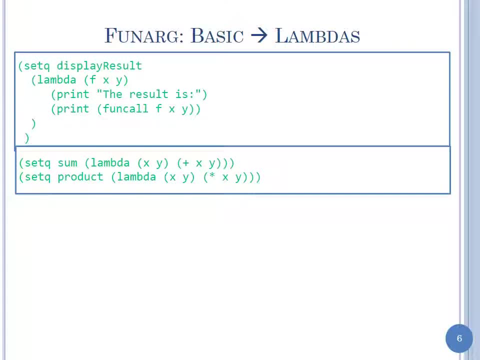 We'll just call it a basic function. Okay, Because we want to pass these things around, So we could do that. Okay, because I don't want to lose this fun art business, fun art explanation. So I'm going to take basic to lambdas. 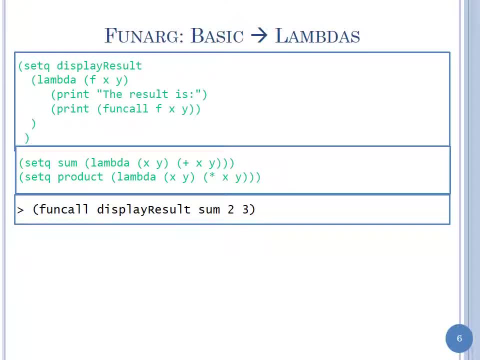 And now if I say fun call, display result: sum 2, 3, sum evaluates to a lambda expression, I can pass 2 and 3 to it And I get what I want. Okay. So again going back to assignment number 3,. 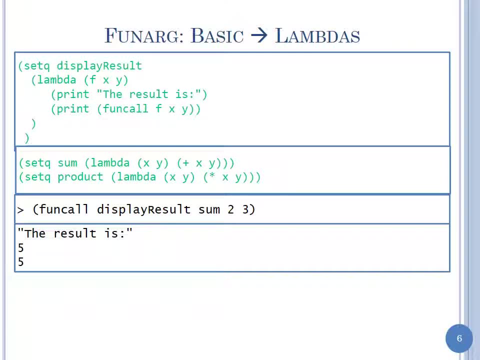 the first part is going to go through this. I'm just going to make you guys do steps like this. Okay, Okay, Func law display result: product 2, 3.. The result is 6, 6.. Okay So. 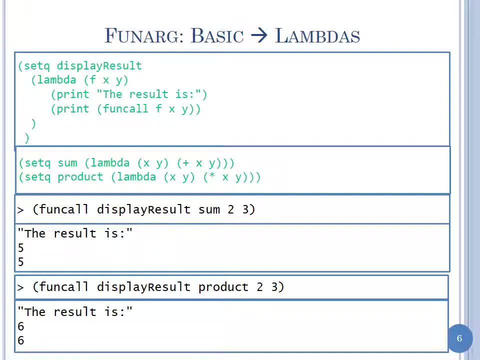 does this remind you of anything? Anything you've done in 401 or even 110-like courses, Passing a function as an argument: Map and filter. So what can explain that? Will you learn this thing? I mean, I didn't take 110 here. 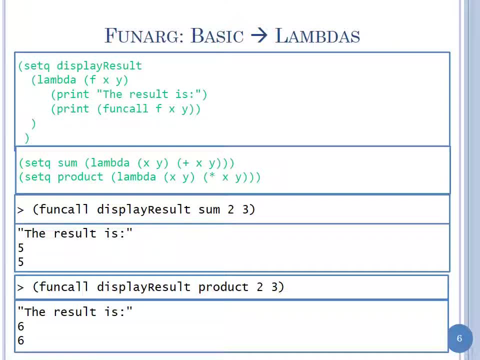 but I know they use like filter-back-reduce and 110 now. So you can like you can pass an array and you can filter, or you can pass a function to a map, like you can square all the elements or something like that. 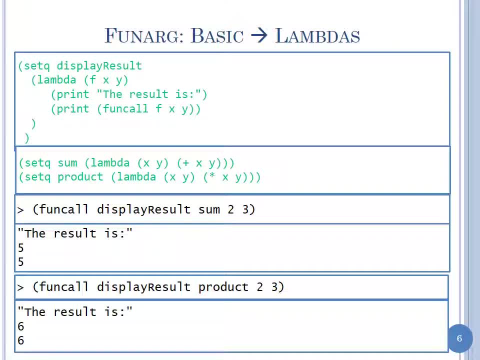 Okay, So that term comes from a list called map-car. Okay, And so that's good. So okay, So then they're doing some functional programming there, And that's good. But how about something that was not introduced as functional programming? 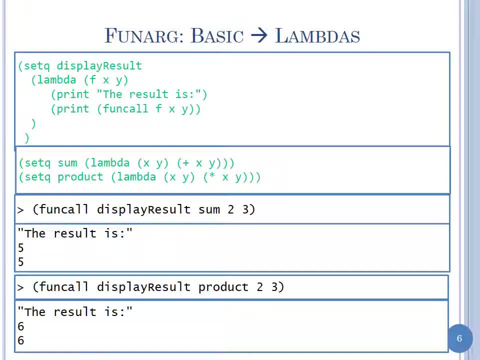 that you just had to do: Yeah, Okay, Passing a class or an object that you made yourself, Passing a class, Passing a class to passing an object? Yeah To yeah Okay. I was just wondering about that. But so when we did, we did like quote a class, for example. 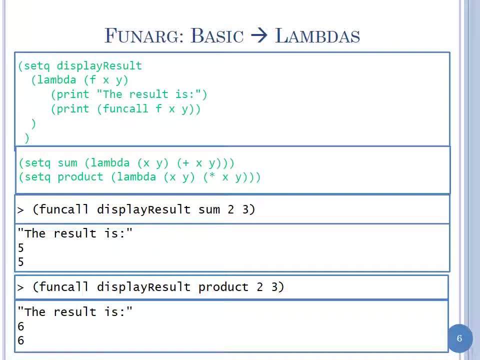 would that still work for the value of the class? But you need a lambda expression. finally, You just need a lambda expression. Yeah, Yeah, You need. so it's just not bound to. Yeah, So you could make a list. 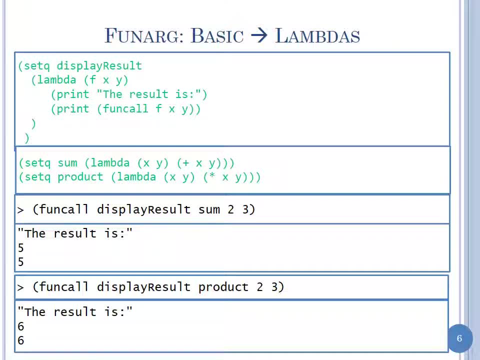 You could make a list with plus as being the first element, And so you could do: if you do a list and you do a code plus and then pass the arguments, then that would be a. you could basically make a call like that: 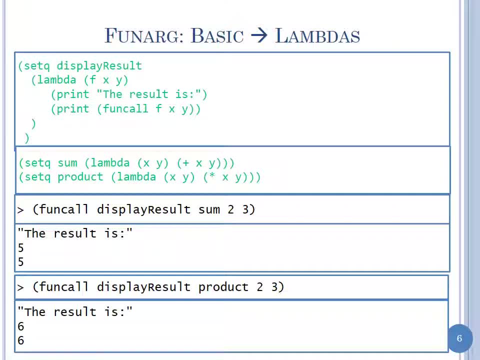 That would work. That could work in another way, not with fun call, but that could be used to go with reuse. That's what I'm saying. list: Yeah, you can make a list with code, so just bypass the lambda part. 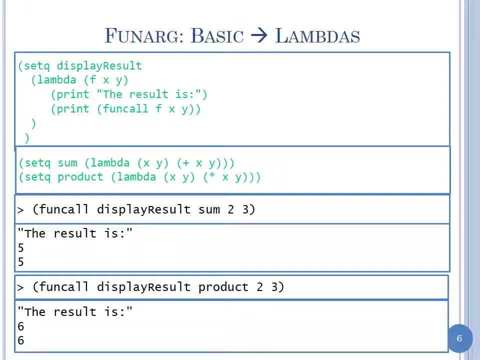 Yeah, that's good. I'm glad you guys are thinking this way. Right, but you're not calling fun art. Fun art will still go in. Fun call- Yeah, you're not doing fun call, Yeah. yeah. yeah, that's a different way of doing it. 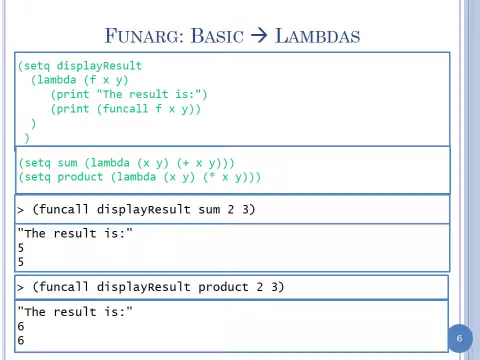 Yeah, Okay. So think of model view controller. Do you see any sort of similarity to model view controller? here There's separation of concerns. Often a model can work with multiple views and views can work with multiple models. Okay, so you try to separate things out. 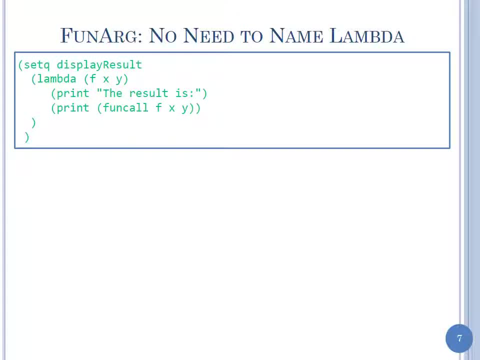 Okay, so before I do that, I could have done this also, by the way, I could have not had, I could have just said: fun call display result: lambda x, y, Something like that. I didn't have to go and name that function. 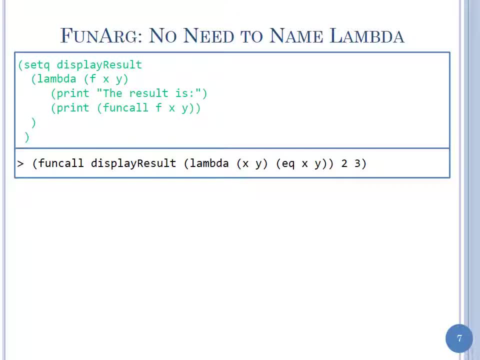 I could have just passed the lambda expression directly to my display result Without naming it as plus, as sum or product. Okay, I could have just passed it. So the important point here is lambda expression. Okay, And I get back something like this: 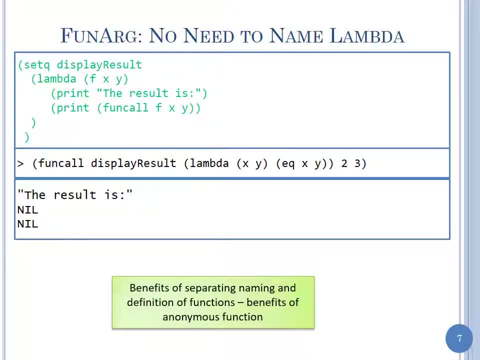 So benefits of separating naming and definition function. So here, what I want to bring out is that you know, when we first did lambdas, you guys weren't modeling. I mean, why are we separating out the lambdas? 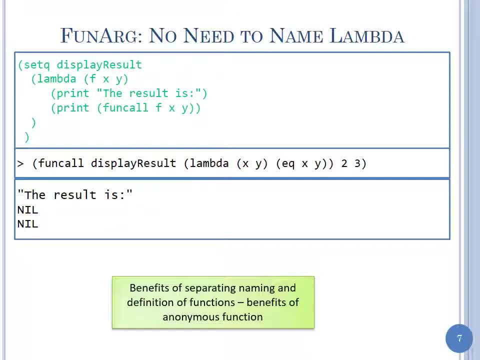 Why are we creating anonymous functions? You know the whole idea of lambda is you can create anonymous function and name it a separate function. When would you use a body without a name? Here I'm using lambda expressions without the name, So this is the first real use of a lambda expression without its application. 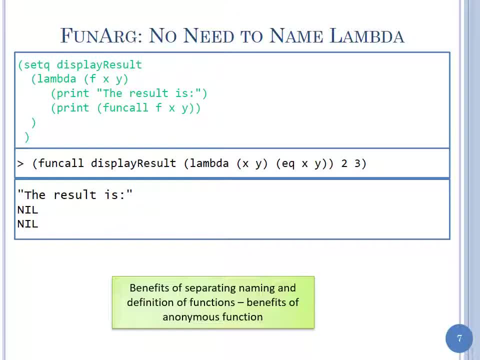 Normally, what we've done is we've defined the lambda expression and applied it in the same line- Okay, Which is not so motivating. Here I've actually taken a lambda expression and passed it to my display result- Okay- And passed it to another function that does something with it. 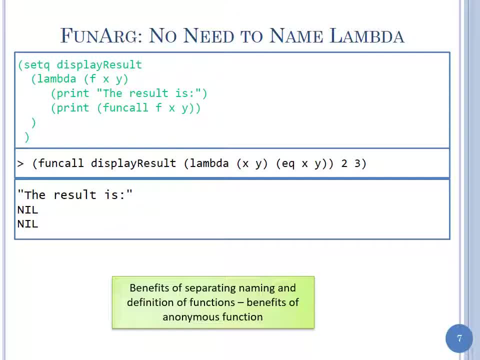 Okay, Without having to name the lambda expression. Okay, And this is typically how lambda expressions are used in Java also, Like when we use a thread example, we went and passed the lambda expression to the thread constructor because we didn't want to name that piece of code and the thread constructor. 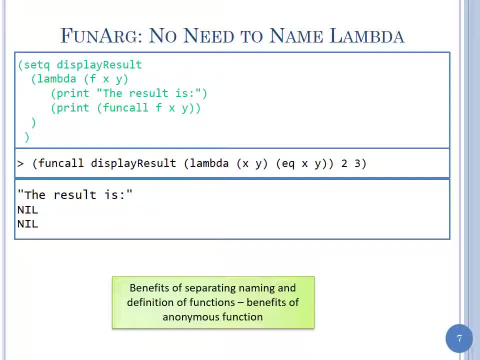 just needs a piece of code to execute. So we went and passed that Okay. So this is sort of like I said, showing you. I'm not saying I'm encouraging you to start a program, Okay, But I'm saying you know, if you want to do something you can do it. 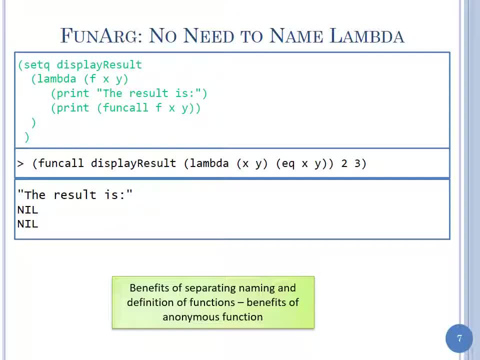 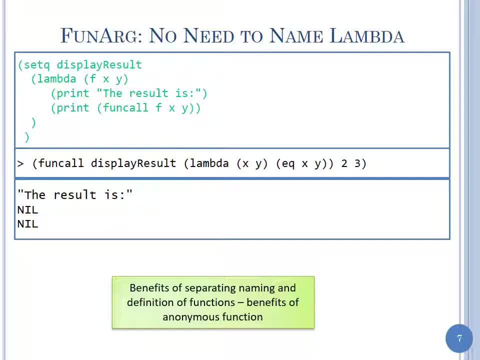 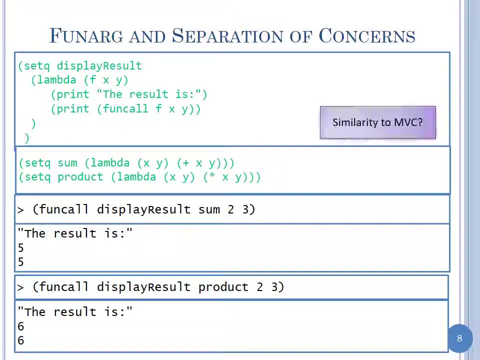 having to name this function. This is a one-time use, So we didn't do it. Okay, Let me go back to this separation of concerns Similar to MVC. So look at this F here F is doing the computation, okay. 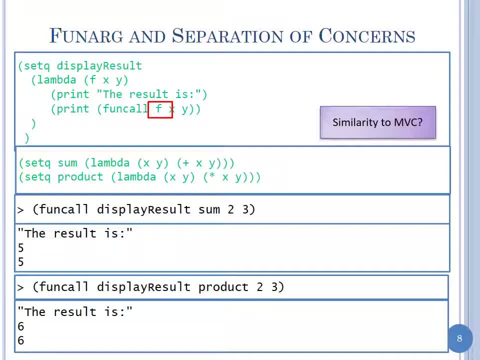 Okay, Okay, This particular function doesn't do any computation. this function is just doing display, which is. and so think of separation of I? O and computation, and what we're doing is that this particular I O code is oblivious to how computation is done. separation of concerns, and we're just 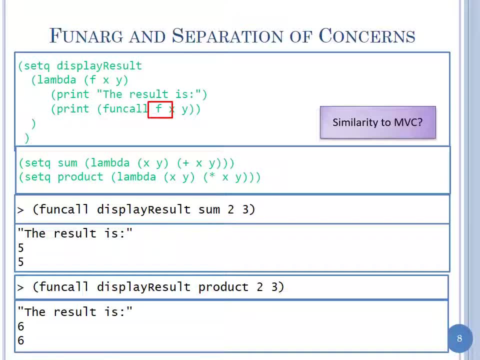 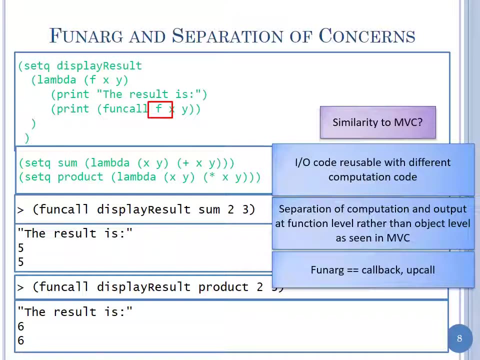 passing that as an argument. okay, and I O code reasonable with different computation code. So separation of computation output at function level rather than at class level, object level, that we're keeping these two things separate. and what I was hoping some of you would say is that this is, like you guys might have heard the term callback- that callback in English. 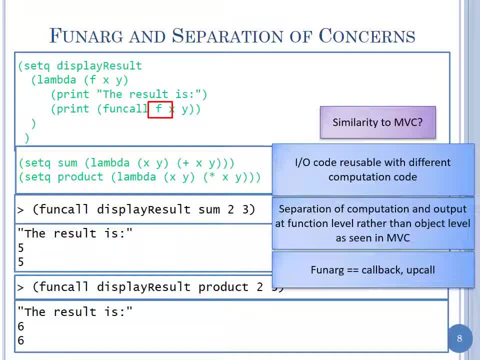 means that you know, hey, you know you don't know me, so I go and call you. I know your number, I give you a callback number and you can call me to finish your task. So a callback routine. typically, if you build any kind of GUI, you build, you create a text. 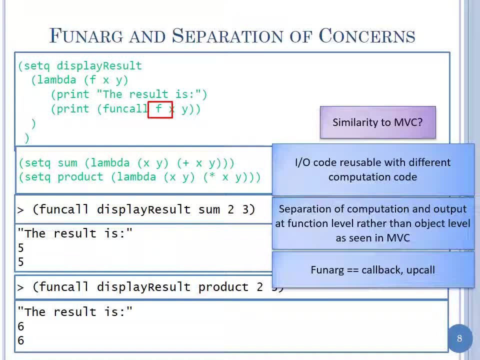 widget or something, and then you want to know when the text is entered. you give a callback object or a callback function which gets called back, and in systems this is something called up call, that the lower layer can call code in upper layer without really knowing anything about it, by being passed dynamically a function that it knew nothing about, which it calls. 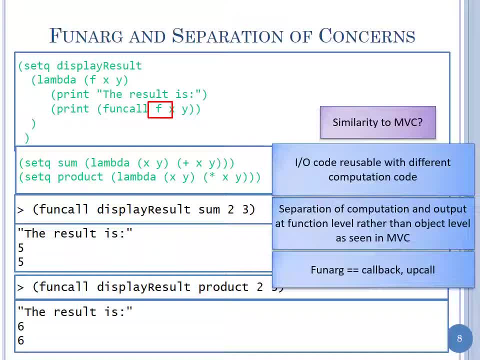 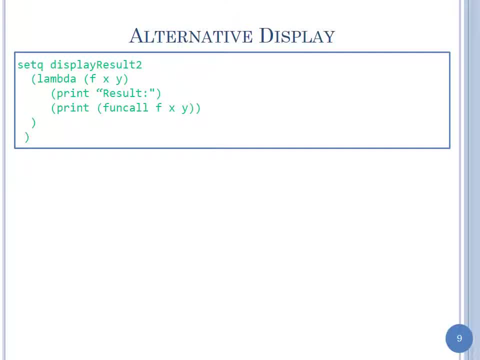 okay, so this is not as alien as it might seem. okay, that you the whole idea of passing functions. okay. So, and just just to complete this thing, I can have another display, result, which displays things separate in a different way. so I am now saying result, colon, and and using the 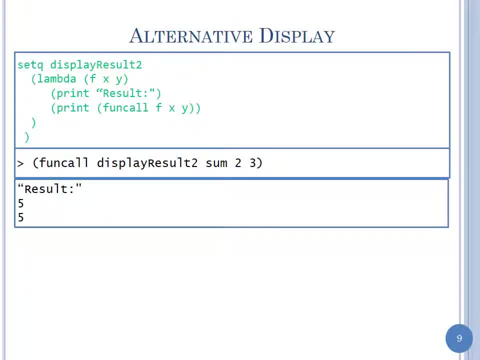 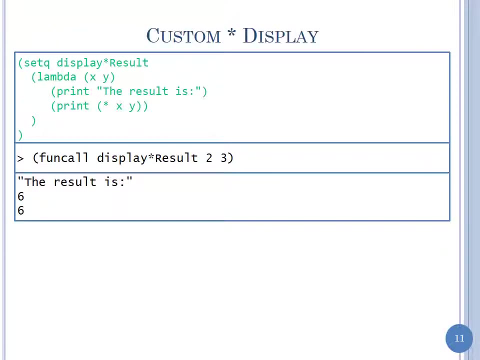 same sum function. so we are really keeping the model and the view, or the computation and the display separate. okay, I'm going a little quickly. I'll review this later, but I just wanted to make this point before we end. So what we're going to do today, 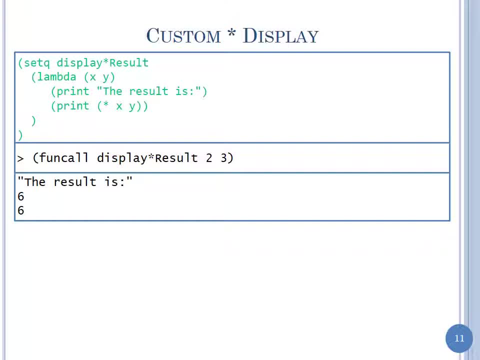 Okay, And in the first part of the third assignment is is sort of the heavy lifting with functional programming. okay, and I motivated some of this work by giving you first a function that prints out a result in a customer custom way. okay, so, rather than just relying on the interpreter, 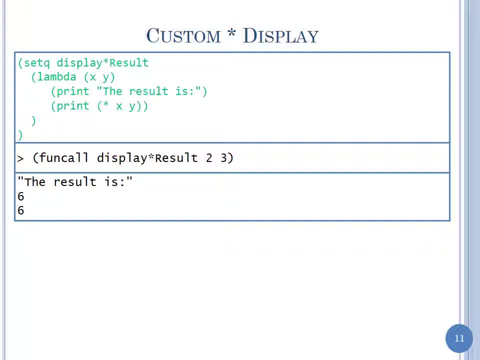 to print out the result. it formats the output and says the result is okay, Okay, And we did that. for multiplication, okay, and we have a. multiplication takes two parameters. so this function takes the same parameters as multiplication does, does the multiplication and then goes and does a formatted output: okay, 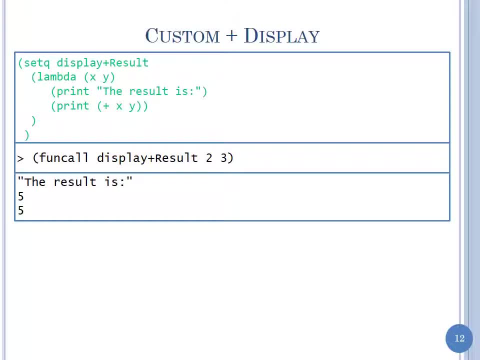 And then we did the same thing for plus. we wanted the same kind of format, uniformity, but we wrote the same thing. Okay. So we wrote a different piece of code which we just copied and pasted and then and then modify, and we got the plus result. okay, and these two functions on their own are not interesting. 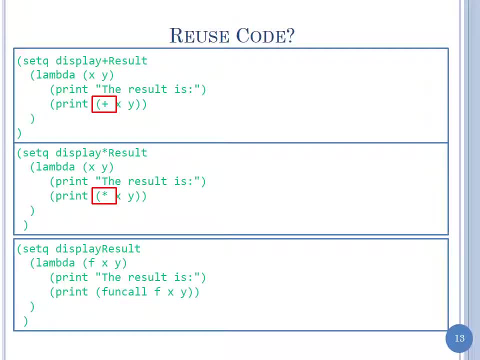 individually. so what was more interesting was how we could get rid of the code duplication. okay, how can we avoid copy and paste? and, and we saw that we could perhaps have a function that takes another function as an argument. so now we have display result and the display. 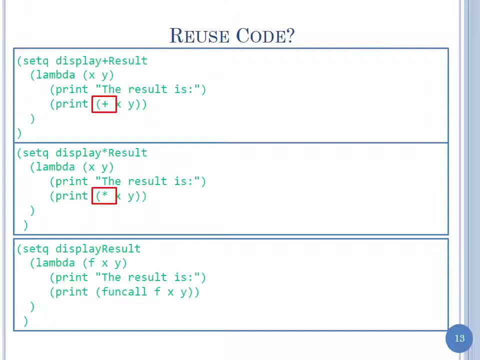 result takes three parameters, not just the x and y, but also the competition to be done on x and y, and that is the f parameter, and it does a fun call: f x y rather than plus, x, plus or star of x, y. okay, So, so this is this was what we, what we did. 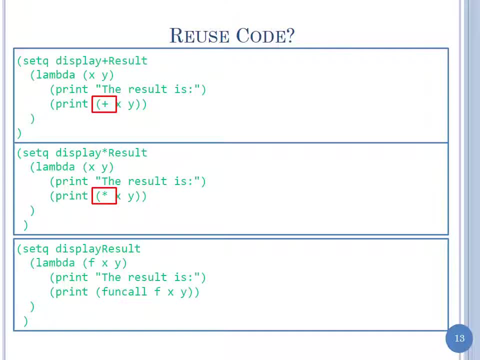 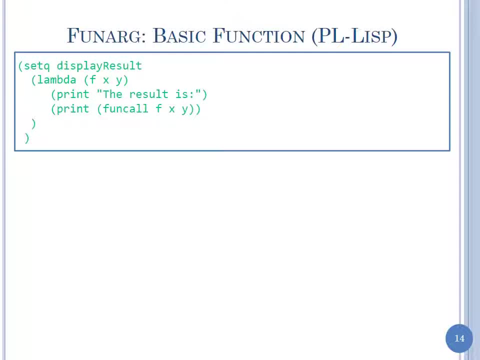 Any questions? Any questions on this? so far, okay, I'm just reviewing. So this is a fun arg, it's a functional argument and here's how I'm calling it. so I don't, I go, I go. so here's how I could try to call it. I could do fun. call display result plus. 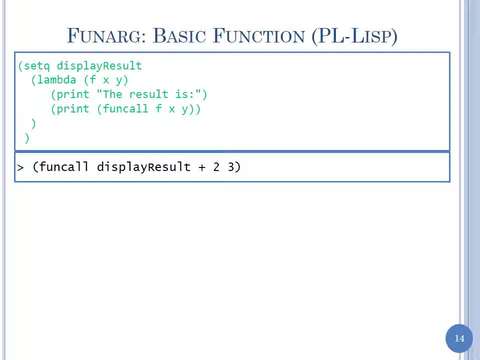 two, three and just pass plus directly, and so we saw there was an error when we pass plus directly. What exactly is the error? So plus is not a lambda expression. that's what we saw said last time, and and and. so what exactly is going to happen when you start to evaluate display result? you're going to 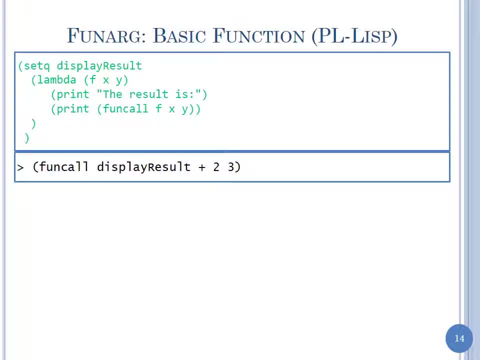 do fun call display result. display result is a lambda expression and what part of our evaluator is going to encounter plus and complain and what? what's going to be the exact complaint here? So when you do fun call of a function, we have the first argument of fun call should be a. 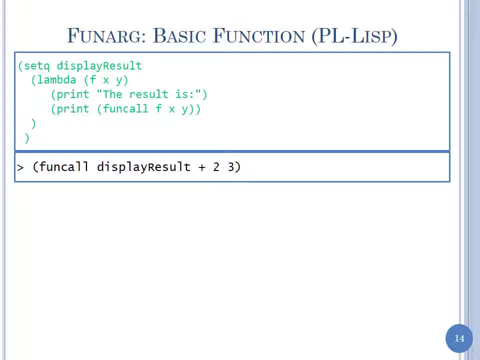 lambda expression, which it is. and then what happens to the remainder of of the arguments of fun call? what happens in the interpreter? what does the interpreter try to do? yeah, so it wants to pass them as parameters. but before it passes them as parameters, what does it do with them evaluates? so it's going to try to evaluate two and three. that will succeed. 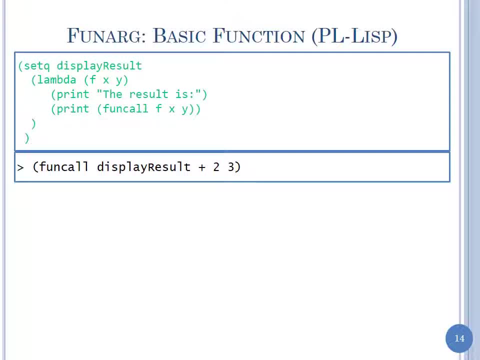 but it doesn't even reach two and three. before it reaches two and three, it has to evaluate plus. plus is an identifier, and what does the evaluation function do for an identifier, but in general an identifier? eval does what, It does what, It does, what. 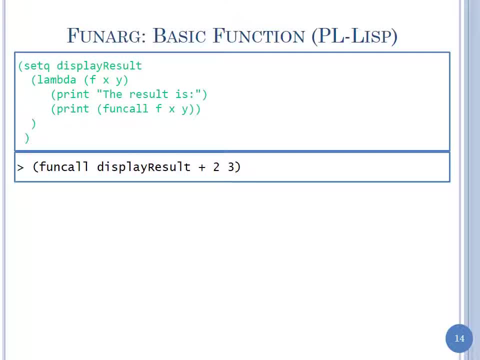 It does what? So was it related to the value? So no, no, that is when plus happens to be the first, first argument in a fun call. that's true if I was to do plus, two, three and plus was the very first element of the application. 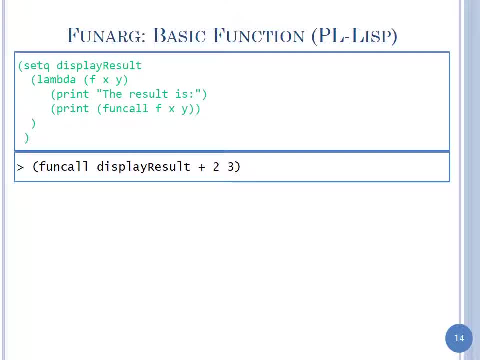 it would go to the evaluator, absolutely. but now I'm doing fun call display result. so fun call is the evaluator, okay, and we expect, fun call expects its first. you know, fun call expects, in this case, display result. to be a lambda expression, which it is, and what does it do with the following things: 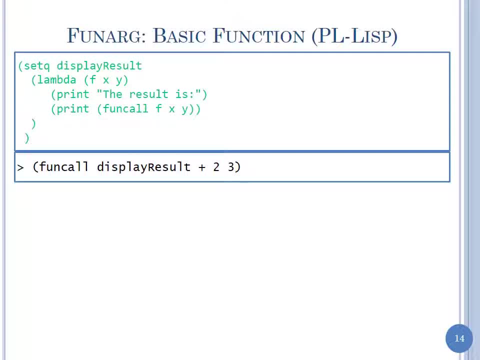 it tries to pass them as parameters of the lambda expression and and it tries to evaluate plus and, in general, identifies evaluated by lookup. okay, so it, you try to do a lookup and there is no. there is no plus in the environment. okay, plus is in your registry. it's not in. 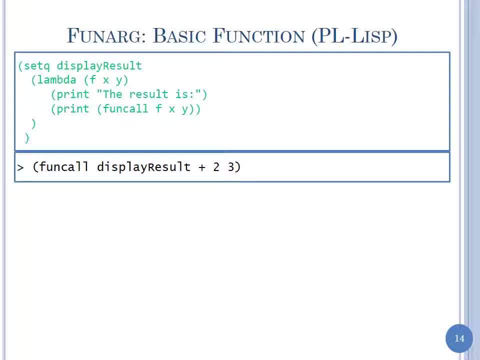 the environment. that's what our list interpreter does. okay, so we'll get. we'll get something like variable plus has no value. okay, we're just saying that. look, I went to the lookup table. I found no value. this is what Andrews interpreter will give me. okay, so we could. 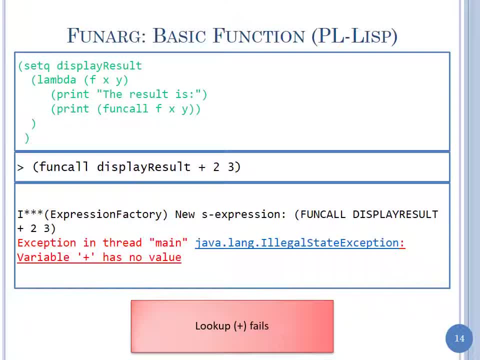 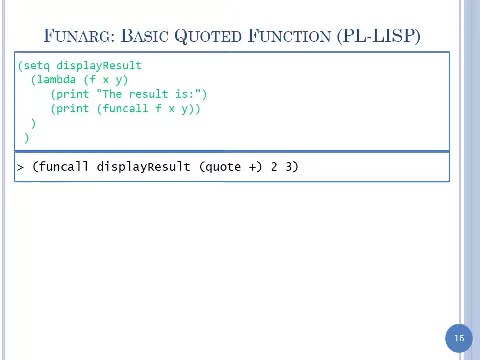 try. so lookup plus fails. okay, so we could try. so lookup plus fails, okay, so we could try. so lookup plus fails, okay, we could try doing this now. try not to go and evaluate plus. you can say code plus and so now my evaluation will succeed. my code eval will return plus, okay, and then what error? 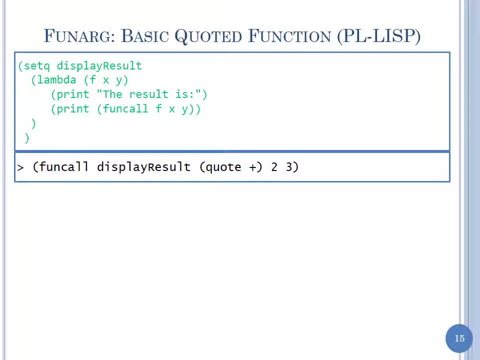 will. that will I get. now it's a little louder, not a lambda, exactly okay. and then, what error will I get? now it's a little louder, not a lambda, exactly okay. so argument to fun call must be lambda, okay. so, yes, we indeed made a mistake by not. 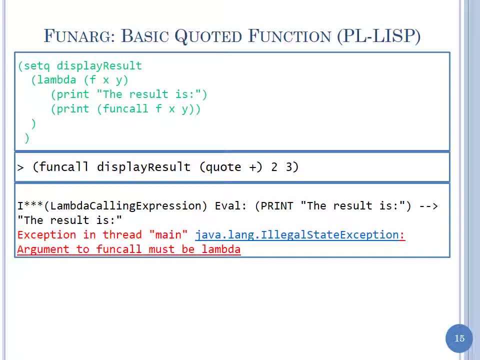 passing a lambda expression there and, and this is, this is sort of the. this is what we get with the interpreter as we have described it in plus. okay, this is not what you get with c-lisp, as it turns out, as I found out this morning when I read Ben's message. okay, so if I try to go and pass this to c-lisp just to see if I can get it to c-lisp, okay. so if I try to go and pass this to c-lisp just to see if I can get it to c-lisp, just to see. 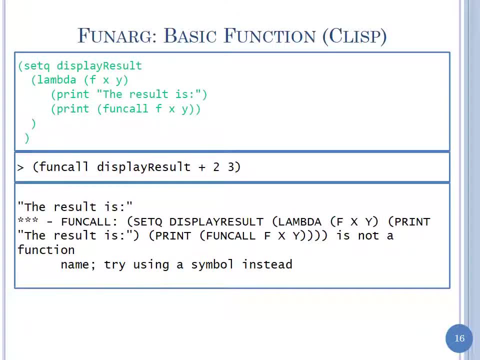 if I can get it to c-lisp, just the plus, that does fail, but in in a way that I don't understand. okay, because we don't know what it's doing. it says print fun, call f xy is not a function, okay. so it's trying to do something and it makes some assumptions about, about what, what. 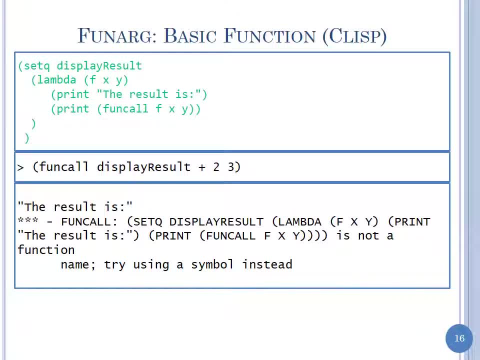 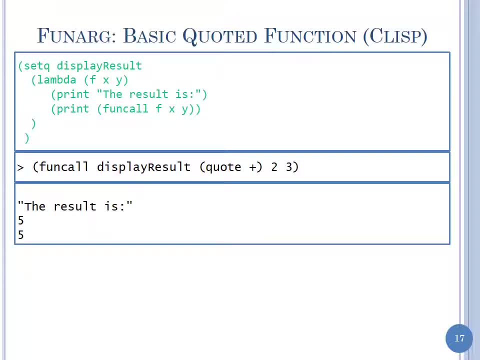 to expect there and it fails, okay. but when we go and quote, it doesn't need succeed, okay, and and you guys can make your phone call, it's good, okay. so we have done that, we have it. but to the c-lisp tool: we have to look at the읛. let us use the c-lisp, okay, let's. 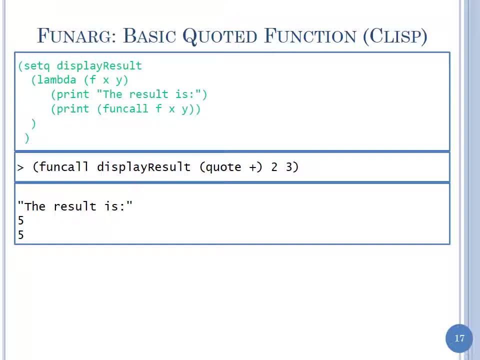 succeed too. you can just go and look at the next parameter, go and see with an identifier. if it's an identifier, do a lookup. if not, do an eval. okay, so you could indeed- uh sorry, not do a lookup. so much as called the basic evaluator. so you can, you can go in. 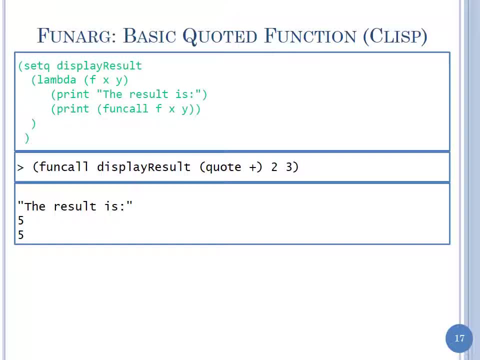 because plus will not be looked up there. so you can go and actually, uh, do what the base, what what you know? look at the, look at the evaluator and pass it to the plus evaluator. uh, if, if the value exists, okay, so you can indeed do that. uh, but that's not what we. 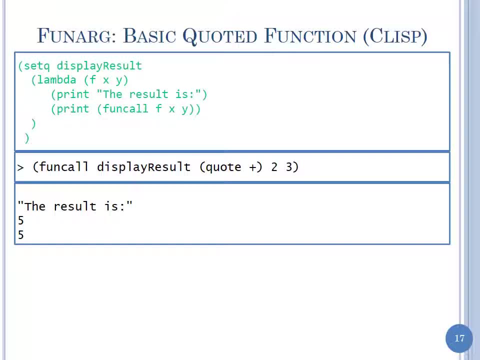 require you to do so. you know, i keep telling you that the list we are doing is not identical to the lisp c-list for various reasons, and so there is, there is this discrepancy, okay, questions okay, and this is, you know, this is, this is special handling of fun call and it's practical, okay, and 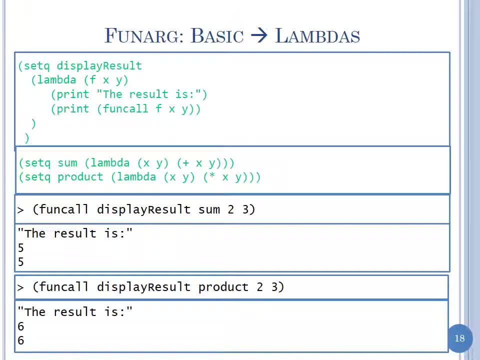 since we didn't have this thing, what we did was we said, go, and let's go and define a lambda plus which we're calling sum. okay, so now sum is bound to a lambda expression and it just takes its parameters and passes them straight to, straight to the basic plus. so we are, we are doing some. 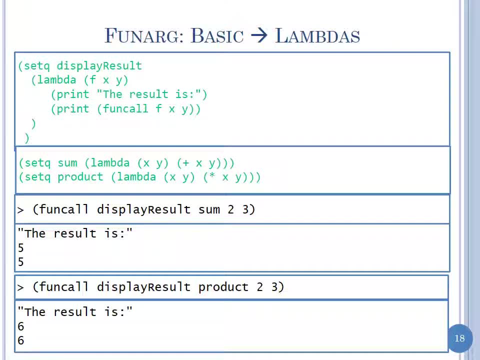 work here, extra work here, and now we can go and pass sum and product to this. uh, fun call and it'll work. okay, so we achieved our goal of reusability at the cost of having to define two different functions. uh, for the basic functions. okay, so your assignment three goes through this process and requires you to do: 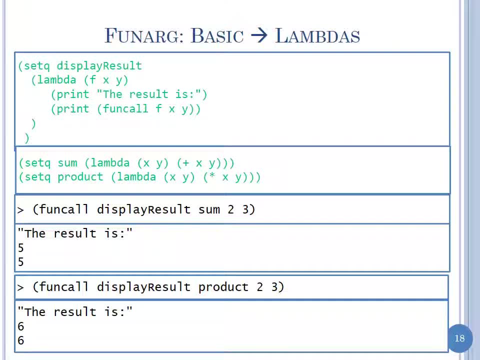 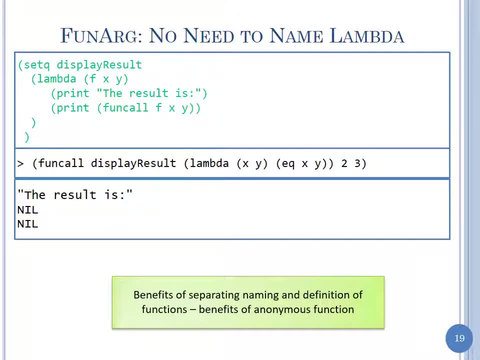 steps. make steps like this, take steps like this. okay, questions so far. and you know, one of the sort of confusing things when i first started lambda expressions was that you didn't see a use for them. okay, yes, you can type a lambda expression and you'll get back. 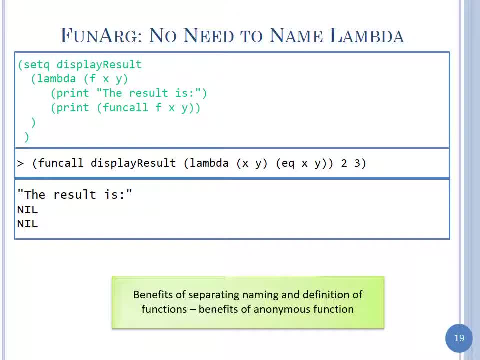 you know definition you did. that's no use. you just wrote a definition and it's printed out and we do nothing else with it later. the second alternative was we take a lambda expression and you apply it to an argument- okay, immediately. so what's the point of having two different functions? 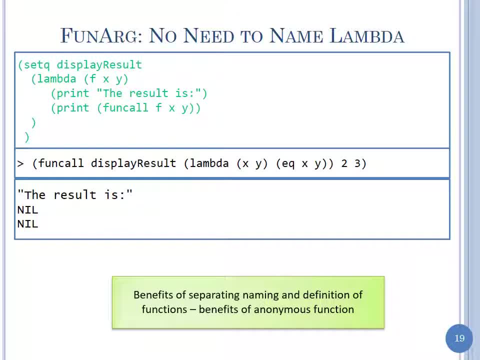 what's the point of having parameterized lambda if you're going to just bind that, those parameters to one set of arguments? yeah fun, you know the, the, the uh usefulness of functions comes from being able to bind different formal arguments to the same, different actual arguments to the same formal arguments. so these anonymous functions. 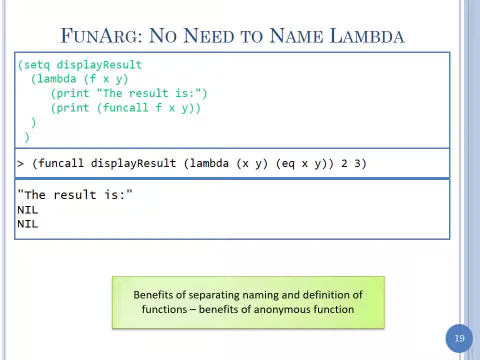 were not very motivated, but you see here now a reason for having anonymous uh functions that i've been using for a long time is that you can have something called display result. it expects the first argument to be a lambda expression. so what i will do is i will not go and define a special 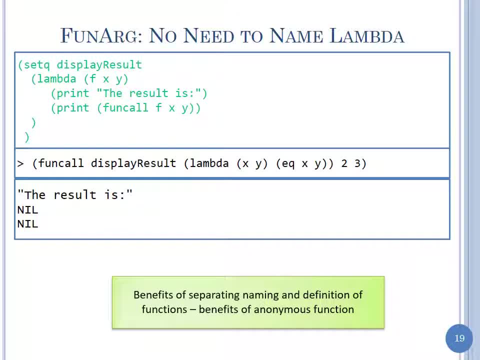 lambda eq. i just go and pass and i won't name it. i just take the lambda expression- not name it- and pass it to my display result and get back what i want. okay, so this is. this is a practical use. i'm not saying this is good programming. 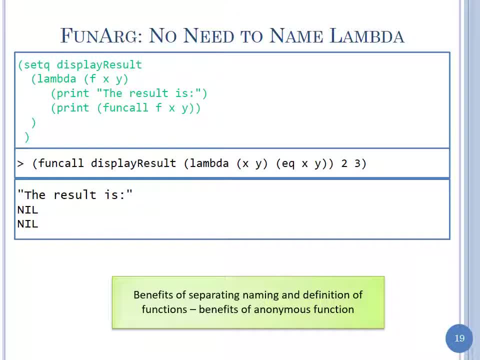 associated with functions, because then i know what this, the function, is supposed to do. so it's like a comment. okay, but if you don't want to do that naming, you just go and pass this, this lambda expression without a name, to uh do something that does require this as an argument and that. 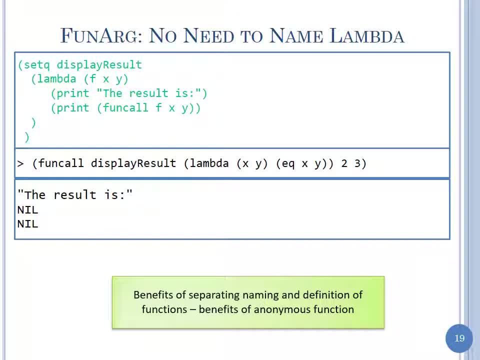 something is going to actually go and assign the actual arguments to its formal arguments, so you will get, indeed, the flexibility you want. okay, so eq, x, y returns nil. okay, because two and three are not the same. so you get the result okay. so, so far, so good. okay, this is yeah. 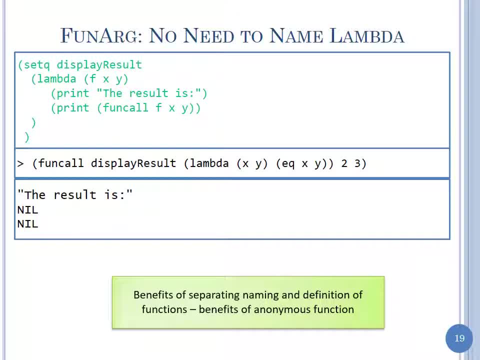 i just want to make sure i understand, um. so basically, the benefit is that you can avoid that problem. if you have plus where it didn't understand and now it knows, it doesn't go into any of those problems. okay, there are two problems. okay, the problem is indeed what you're saying. okay, 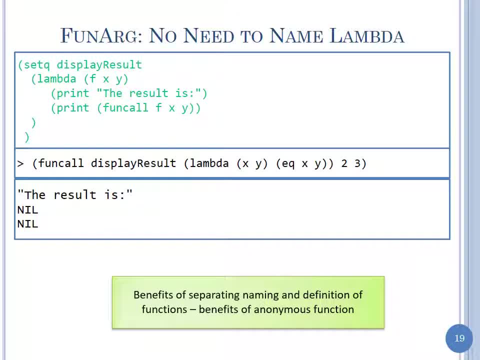 that i didn't. i eq is another basic function and i don't have to go and define a lambda eq. okay, so sorry, i need to have a lambda eq, so that's. that's a solution that i need a lambda expression. once you have lambda expression, the second problem, which is the lazy person's problem. 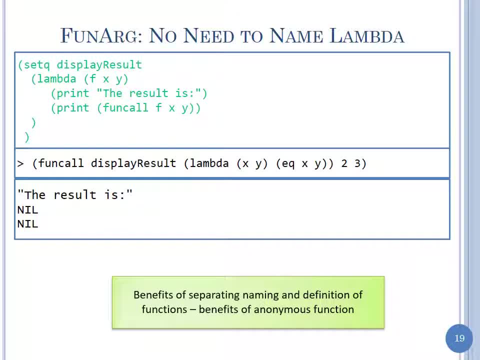 is that. i know the lambda expression. i don't want to name it something, leq or something. you know, i don't want people- people hate naming. okay, because we don't make sense of it. okay, just as people hate commenting and commenting, you can write. you can write some stuff and nobody will look at it later, probably, but the name is there. 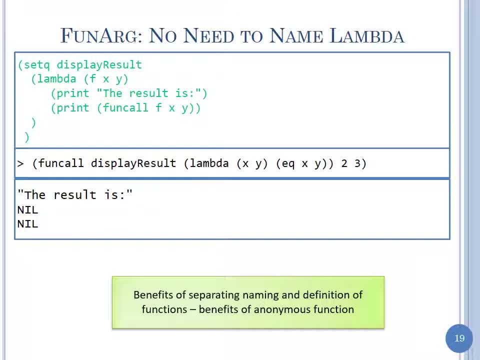 for again and again. so so i'm trying to solve the primary problem of not having the basic eq, having a basic eq and not a lambda, if you. the secondary problem of not having to name a lambda expression, because what we expect is a lambda expression. we can pass the lambda expression. 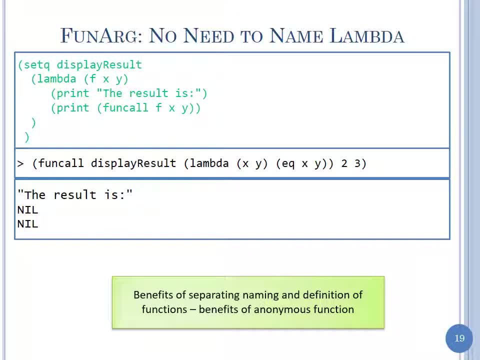 directly. okay, so this is very important. some of your interpreters may not work any longer. the fun call to be followed by a name and you do a lookup of the name, your interpreter will fail in this. but if you indeed go and say, look what follows, fun call is an expression i will evaluate. 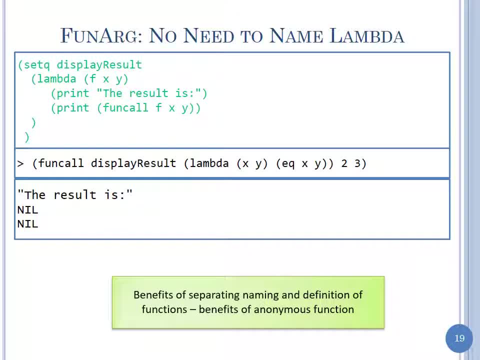 it and i'll see whether this lambda expression or not and then i will go and apply it. then it will succeed, okay, so i know a lot of you guys were doing lookups, at one time at least, and i tried to emphasize in class: this is dot eval. okay, so this is like my um, the use of lambda expression. 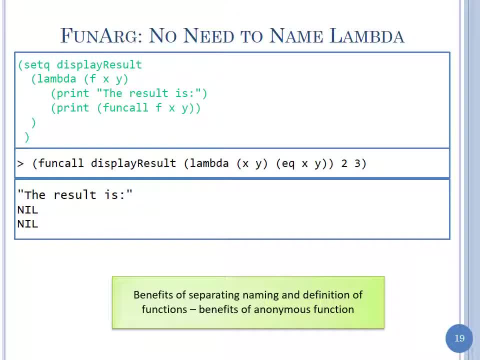 in creating a thread when we looked at java threads that i went and just said new thread and i just gave the body of the run method without having to define a method called run. okay, so again, i'm not saying i'm advocating it, part of the reason for learning much of 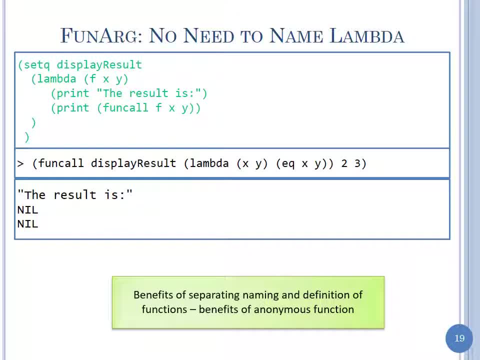 this stuff is to understand other people's obscure code, even if you think that such code becomes obscure, okay. so i personally don't like inner classes. i don't like lambda expression expressions, because i want names. i want names to tell everything. my names are one paragraph long. 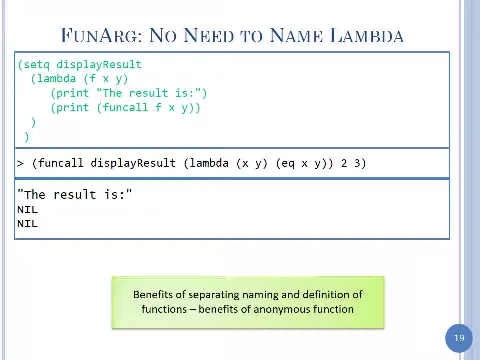 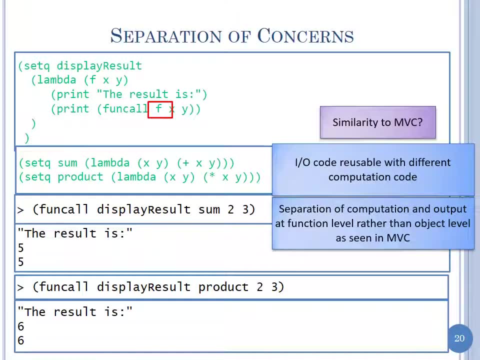 okay, so. so i want those to be descriptive. okay, other questions, and i want to make now pop up this thing: yeah, we're talking about our list interpreter. we're talking about this, but you know, functional arguments occur in all kinds of languages. some handle them more nicely than others. c handles them badly because 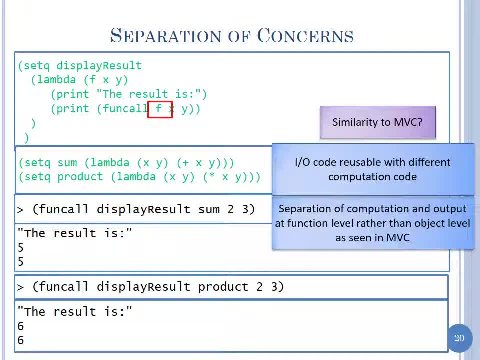 you can just pass it, and this also in substance handles it badly because it doesn't even look at the header of the argument. any function, any function can be passed to a function that expects a function. okay, So I want to sort of say that, you know, with functional programming, not only do, we did. 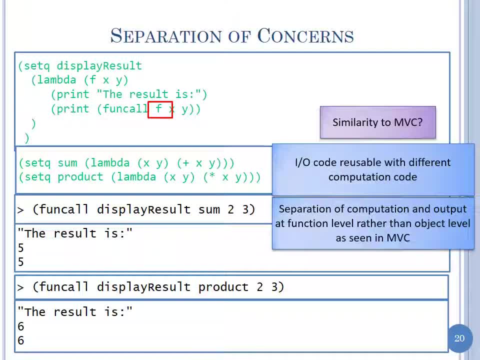 we get reusability. do we get reusability, which is the motivation we had so far? but we also get separation of concerns. okay, and separation of concerns is that if two things are independent of each other, that means one can change without changing the other. let's go and put them in. 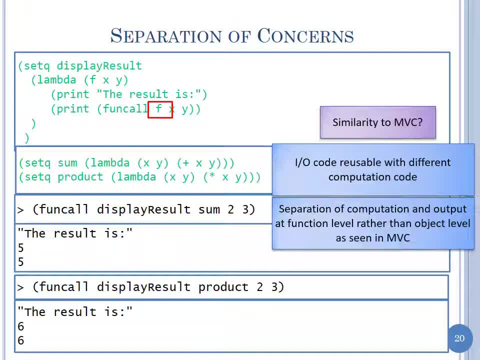 different constructs. okay, in object-oriented languages we talk of different classes. we don't have different classes, let's at least put them in different methods or procedures. So, and the particular concern we have right now is computation and IO. okay, now, there are two viewpoints. one says that computation should be one unit and input and output should. 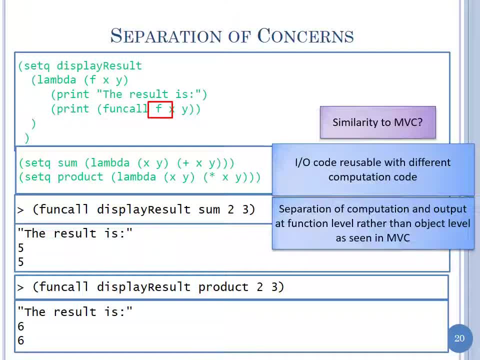 be together, One cohesive unit and the small talk idea which says input should be separate, output should be separate and computation should be separate. okay, so three, two levels there. So here I'm sort of combining the input and output and my display result is just it's. 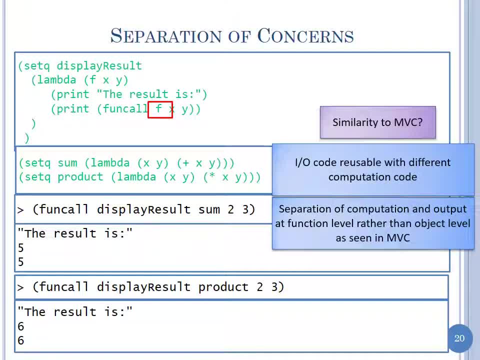 like the controller too. it's calling the function, plus it's displaying the results, so it's doing both the controller and view job, but it's not doing any computation. okay, and it's not hardwired to a computation. the computation is something that's a parameter. 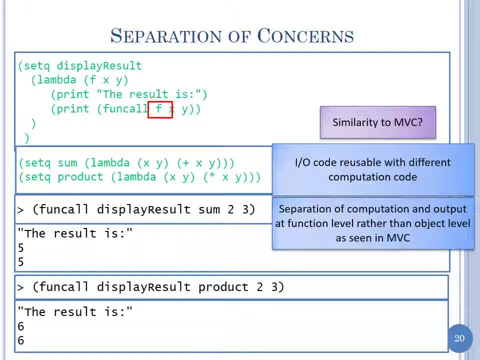 To this and the same view, if you will, or the same IO can be used with different functions, different computations. okay, that's what we have here. display result can be used with the computation that sums and display result can be used with the computation that that. 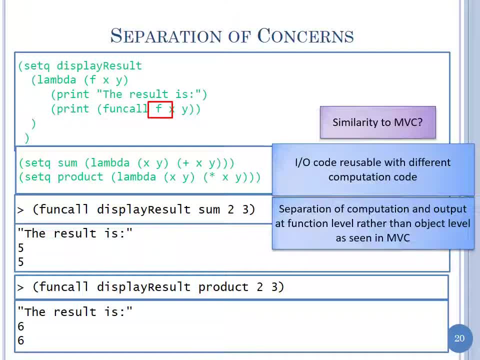 that, that that multiplies. it is oblivious, it's ignorant, unaware of the exact computation. okay, so I'm just trying to drive that point. that that's one reason for having- Okay, You know, functions as arguments. okay, and not only that. so we have same IO, two different. 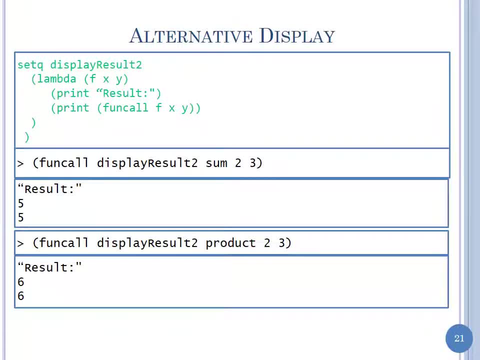 computations so I lost the recording there. so I used last time the term callback and up call Okay for a function, For a function being for a function parameter, And we kind of motivated callback at least. so why is a function parameter call the callback? 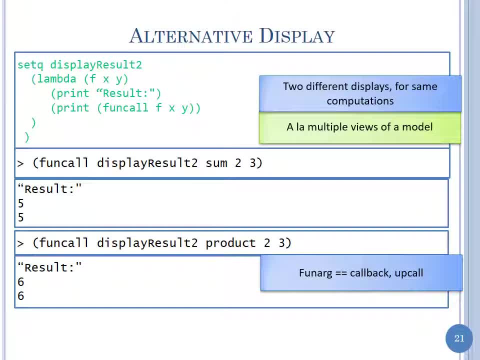 Okay, so, so, okay, so, that's good. you call the first function and that goes in calls the parameter, right? why don't we just say it's a call? why do we says a callback? it is a form of call, right? so why do we go and qualify the call as a? 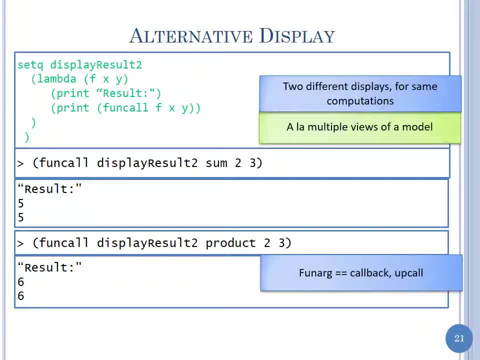 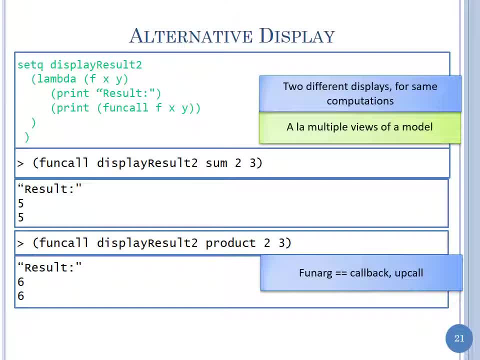 that in the english language. what do we say? i, i leave a message on your answering machine and say: call me back and here's my number. you get a junk car, right, you don't know about them. they know about you, unfortunately. and uh, and they leave a number. you know fbi is after you call back, so uh. 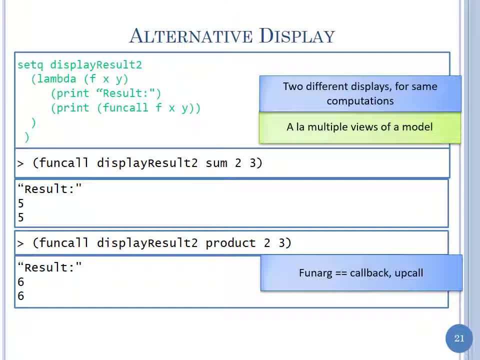 so, uh, you may or may not do that, but so, so that's the unaware, okay, and why would you call it a call back? why? why would you, you know? so i'm saying it's also it, it's called callback, it's also called from a software engineering point of view in some context. okay, and you know, somebody else want to. 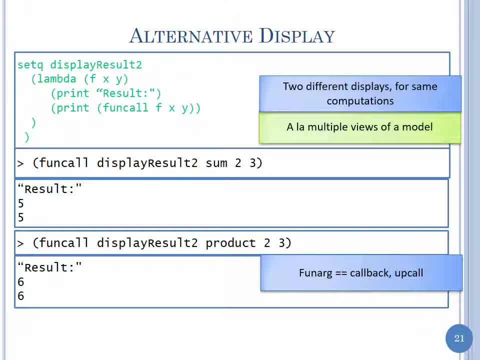 raise your hand. that before i. why would you call it up, call and what is the word up and down going to be relative to? okay, mac, maybe the stack stack. okay, so that's good, that's a layered thing, uh, but stack stack is a, it's a dynamic thing. think of something that's. 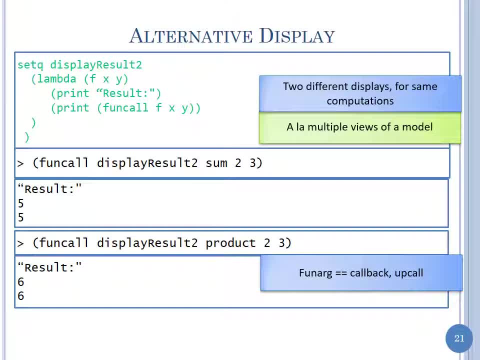 got these levels at at program writing time. yeah, higher memory location. but you know, virtual memory or physical memory. it reminds me of monty python: african seagull or european seagull? uh, you know. either way, you should be quite oblivious of where memory is, you know, especially if everything is in the heap. 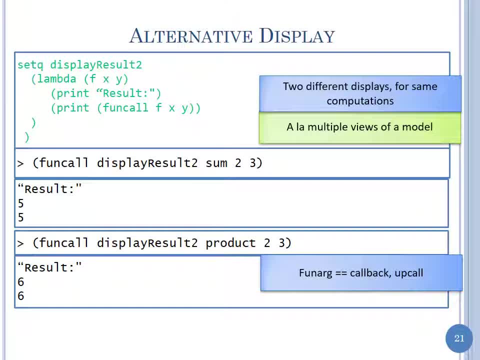 you just don't know what's going to be there. so, but indeed, higher virtual memory is code and data, but uh think software engineering. i'll take nathan, but nathan, okay, i think it's because if you're, if i'm listing off the functions in like a tree style, you would like. 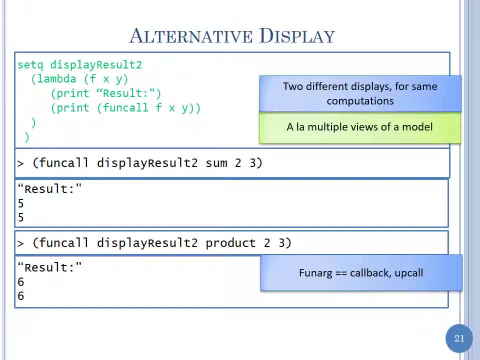 open the function, see what's in it, but it's on function that would be higher in the tree. so it's like like, if you think about like tabbing, then it's calling function of the different areas. so that's kind of the answer, like we got earlier about stack. 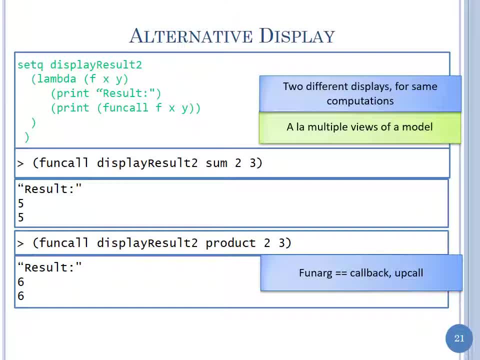 okay, so the stack is sort of the dynamic chain. yeah, but in software engineering, so in operating system, the kernel would be under the client code. so what you say is the kernel calling that code excellent. okay, so the kernel is something given to you and the code on top of it relies on the kernel. so it's. 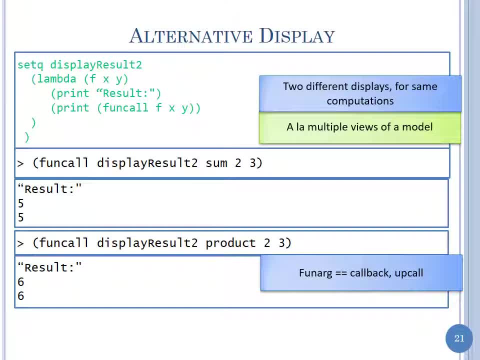 called layering. it's not just operating system. if you're doing networking. there's seven layers, three layers, four layers- who knows, depending on who's written your following- and but in general there's notion of layering. that code that runs on top of the kernel knows about the kernel. 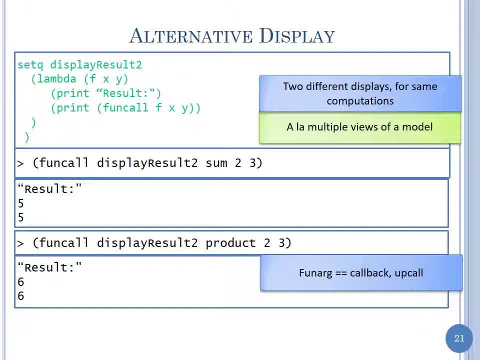 the kernel does not know anything about the code that runs on top. if you want the kernel to go and call something in your code, then that code will be up. it's a very dangerous thing to do. I've seen many operating systems designed that way. why is it dangerous to have a cause in a kernel privilege escalation? I 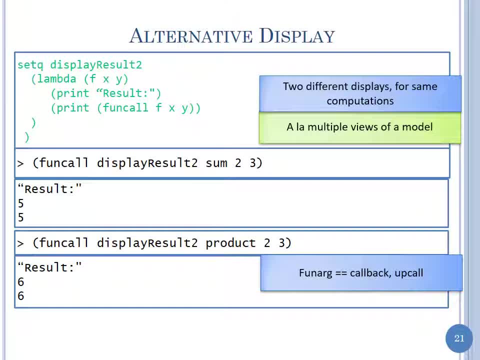 mean, if your code goes in, just has an infinite loop, nothing else. okay, your kernel has gone into an infinite loop, okay, so what they do typically is that if you are like up calls in the kernel- and there was a PhD student whose committee I was on, we did this- they try to define a safe language. you know which? 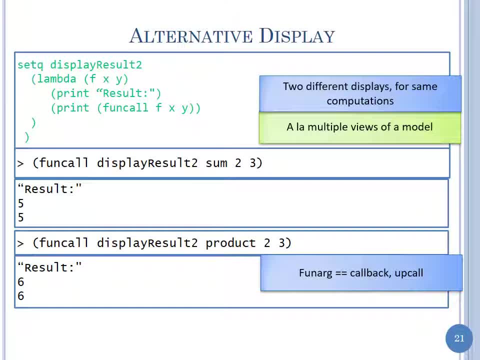 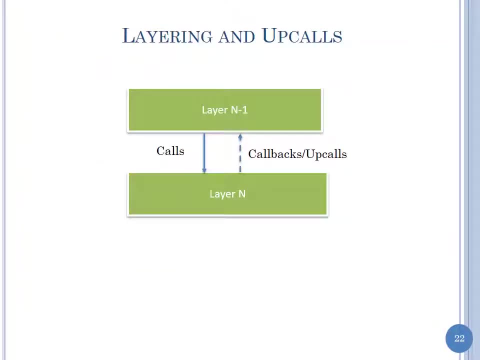 is not hearing complete which can allow you to do that kind of up call. but when you do an intro, when you call an interrupt routine, then some lower level part of the kernel calls a higher level layer of the kernel. so there is that kind of stuff. so let's talk of layering software engineering. so we talk about separation. 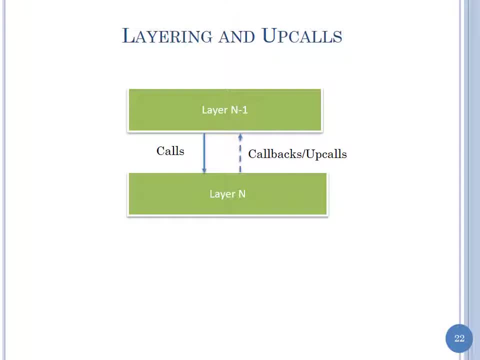 of concerns, that let's go and separate things out. a stronger condition is that these, these concerns, should be layered. and what does it mean? for- I've kind of said it, but that's going to find it formally- what does it mean for some layer to be above another layer? I mean, I can just draw it above. is there a litmus? 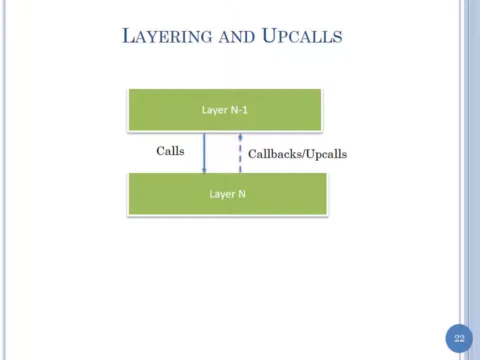 test to figure it out that this layer is on top of this layer. this layer is behind below this layer. yeah, 0, it's got a different scope. that's true in some sense in the region and sense. so if it, if it knows about them. ok, so when you have classes, all classes of these, 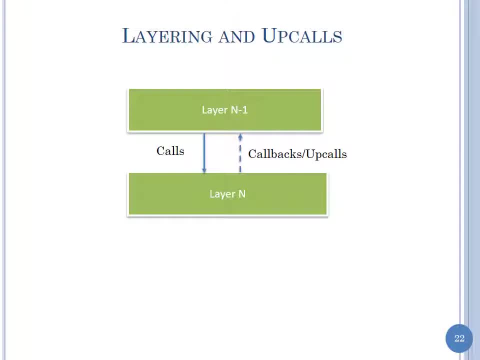 0 at the same scope. okay, the question is: do you know about the scarps classes? are you linked to them or not? okay, so a layer above the higher level layer uses the functionality of the layer below. it, knows the interfaces below it when. so when you are writing that in the higher level layer, you know about the layers. 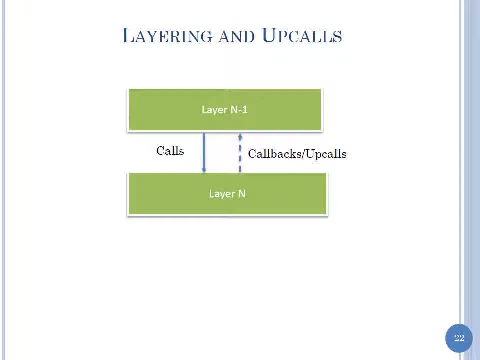 below. you can import something from a lower layer. a lower layer can import from you. so, Andrews, risk interpreter can't import your code. it doesn't even know what you've written. your code can import, Andrews. okay, application program can call kernel routines. that's a standard api. the 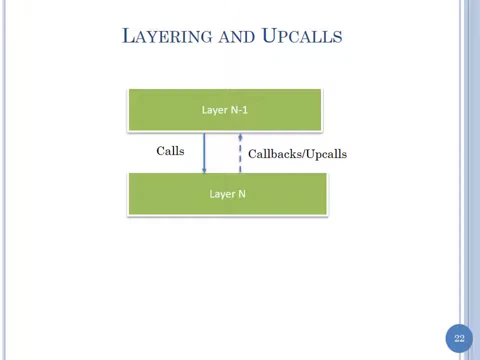 contal can't call your routines. it doesn't even know who you are, you, whether you'll ever exist. okay, so that's layering. and then there is two kinds of layering. can you only call the routines immediately below you, or can you also call the your, your descendants, or i'm from the descendants? 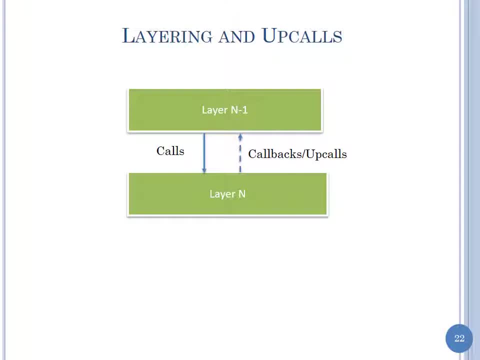 but layers that are, that are not allows any change difficulty. okay, so the calls occur can occur to the layers below you, but up calls can occur the other way around. okay, so the upper layer can go and say here's a function and please call it. you don't even know what that function is, but you call it and you've been told about it through. 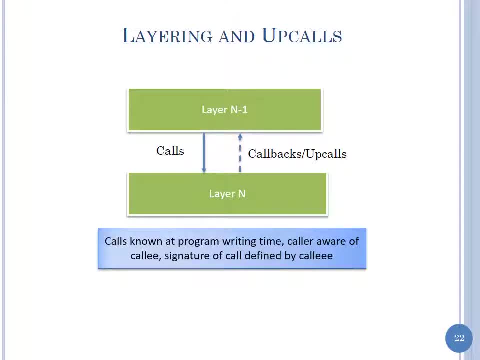 some dynamic system. okay, so calls on a program writing time where the caller is aware of callee and the signature of call is defined by the callee. the kernel defines its api, not the, not the application program. okay, andrew defined his api, not you guys. okay, and you went and called his routines. so if this is what calls are, what are callbacks? 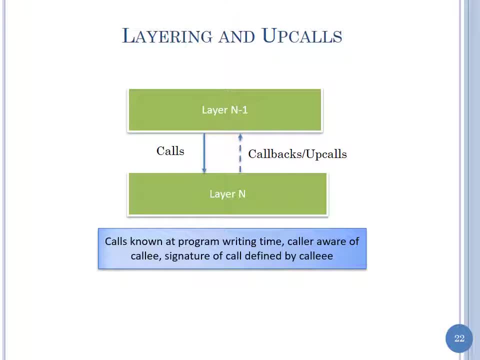 are they known at program writing time? no right, uh, so signatures defined by who? so in in? in a down call it's defined by the callee. in an up call it will be defined by- because the lower level layer doesn't know what signatures you will invent. it defines the signature. it says here's the signature i understand. 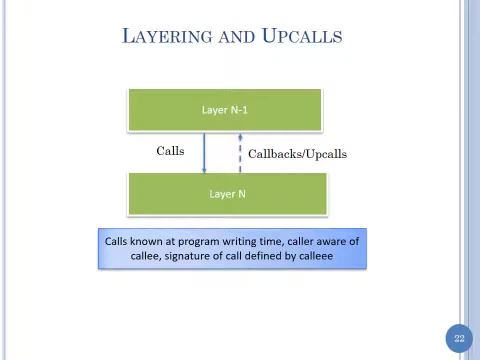 i don't know what the implementation will be, but you better send me a two, two argument function and i'll call it. whether it be product, whether it be some, i don't know, but it's a two argument function. okay, so it's known. at execution time the exact code is known. 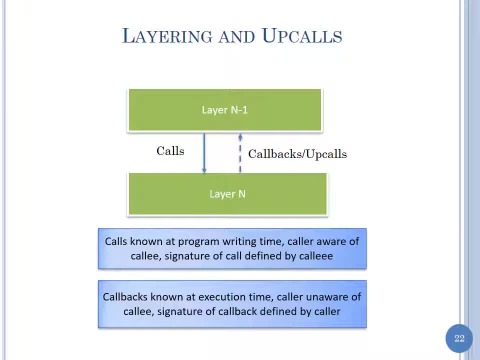 at execution time. the caller is unaware of quality and signature callback defined by column. okay, even in calls. you know, with objectuardial programming it becomes a little tricky because you know the signature, you know the uh calls are known at program time, you know there exists an object of this type, that 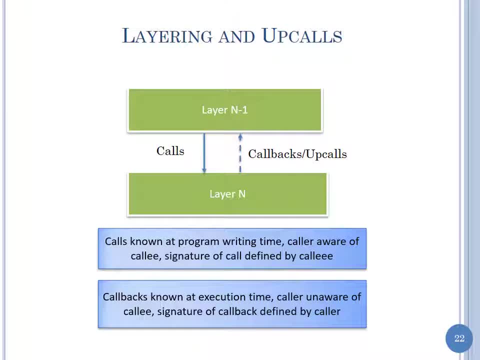 will actually go and execute it, but you don't know which specific type will be used and which implementation will be used because dynamic dispatch- so dynamic dispatch- makes things a little confusing with the call caller thing, but in a language like LISP or C it's more clear that you there is no dynamic. 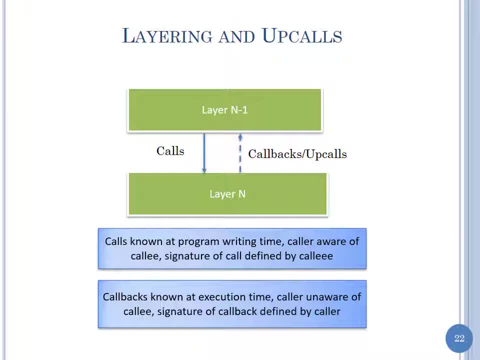 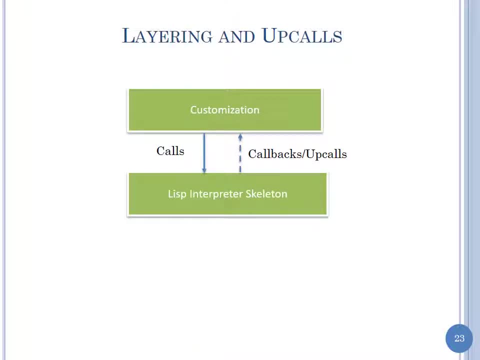 aspects and cons, Okay, questions. so your listen interpreter skeleton and your customer customized interpreter have this cause callback kind of. and this is important because in our, in our system, we wrote this interpreter in Java, so we use java's mechanisms to go and extend it. had i written, had andrew or i, whoever written, 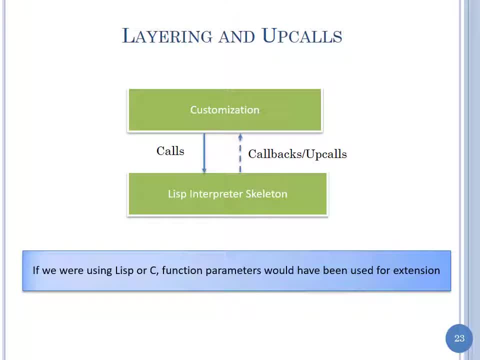 written the list interpreter and see your list. then if i ask you the same question as i asked in the exam: what ex, what capabilities are used to extend it? you would say of calls, or you would say: function parameters. okay, so had we not had dynamic dispatch and interfaces and had we rely relied on 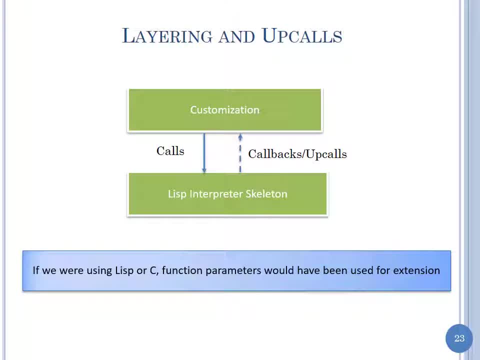 a different kind of list interpreter, then we would have had used different mechanisms to extend header. so header files is the form of, is a form of interfaces, indeed, but the exact. you would still have to pass the functions to the list interpreter. at runtime you can say: here's my functions. 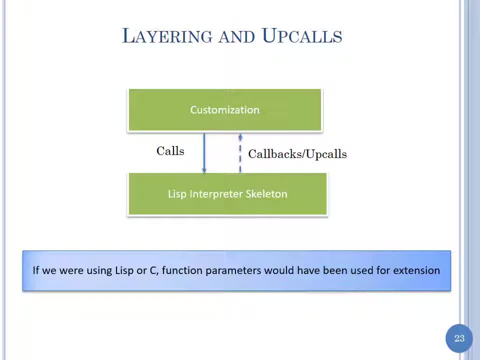 it would not be very type safe, okay, but it would. it would. it could be made to work. so had, like i said, if we change, rules are changed, then the answer would have changed too, because up calls would give you the same kind of customization, extension, flexibility, okay. questions. 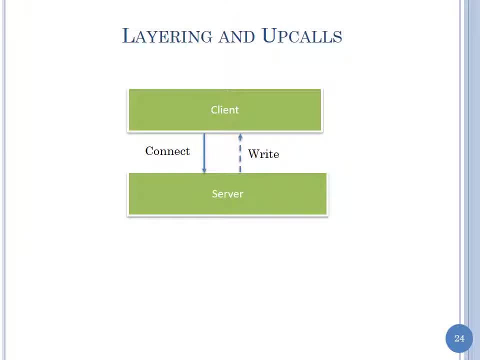 can you see a connection between the distributed server client, and i mean, i'm kind of showing you the connection. so why, why, uh, why is interaction with the server a call like thing and why is the interaction between the server and the client an up-call like thing? 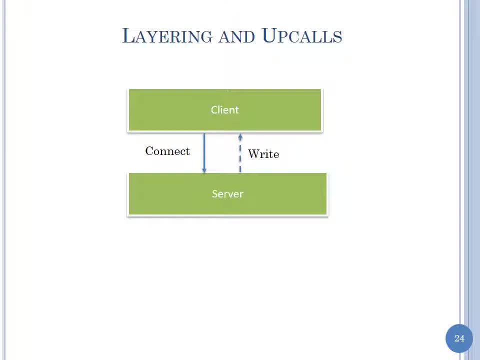 Were you raising your hand. I wasn't sure whether your pen was up or not. Servers are known and names and clients are not known. So servers are known. That's what we said. If there are two processes, they're talking to each other. 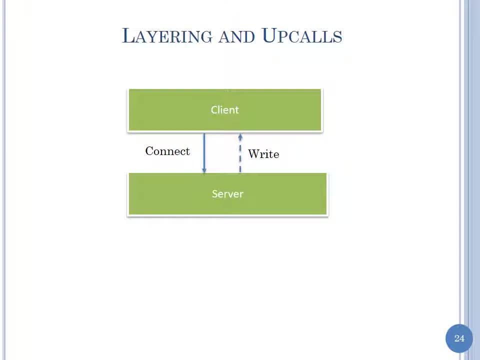 which is the server, which is the client. we talked of one-to-many, many-to-one kind of things and when I taught this to a student, one student said one is a dumb thing and one is a smart thing And basically it is a. 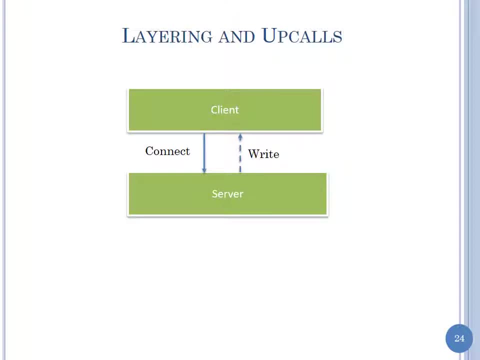 the client knows about the server, Sends its host and port to the server and it doesn't connect. it says here's my host and port. This is all done underneath, you don't really see it. And then the server calls back or sends messages. 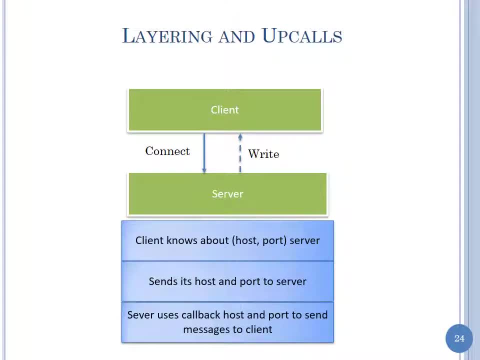 based on what was sent at runtime. So the same general principle, if you will, they don't call it up. calls and calls, but if you think about it abstractly enough, that's what's going on, And server came first. so that's what you're layering yourself on. 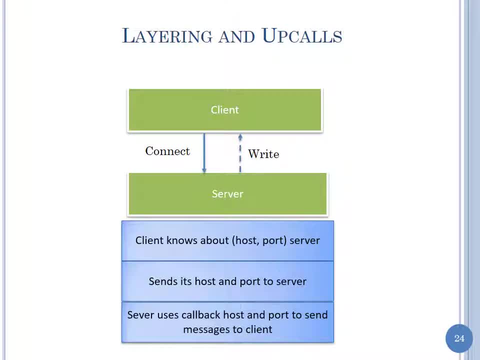 The client depends on the server. The server doesn't depend on what was written in the client. In fact, a lot of times people go and replace kernels. so when you want distributed operating systems, you make the kernel be a distributed agent So that you can make API calls. 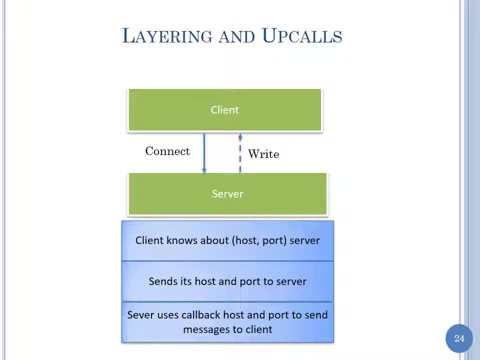 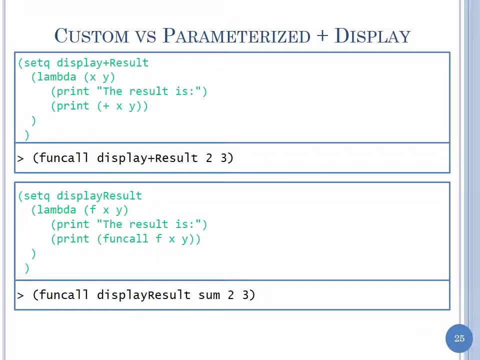 essentially to another computer. So these are very related concepts, Questions. Okay, So let's have. let's look at what we had. We started the display. We had a display result that was kind of bound to plus. Then we came to a display result. 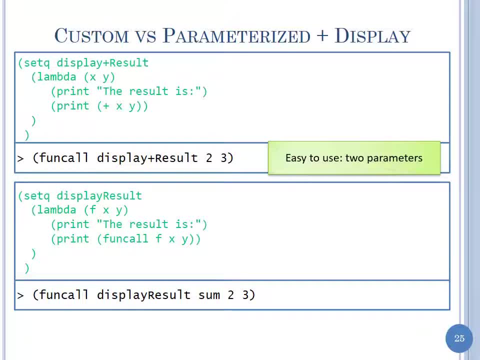 that took the function as a parameter, And what we ended up. you know we were duplicating code. that's bad, of course, but you know the call was easy: We could just have two parameters, whereas now we have to pass three parameters. 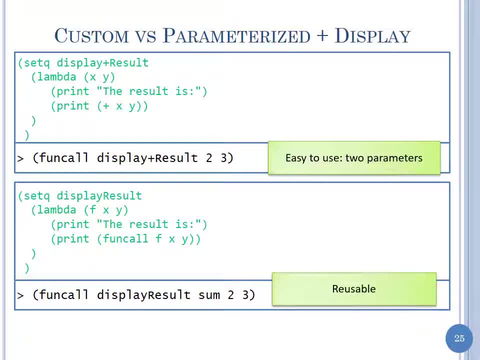 Okay, but it's reusable. So can I write a reusable piece of code or reusing code that takes two parameters. So can we rewrite display result, display plus result to, and this is not a very subtle question, but I'm trying to lead to something else. 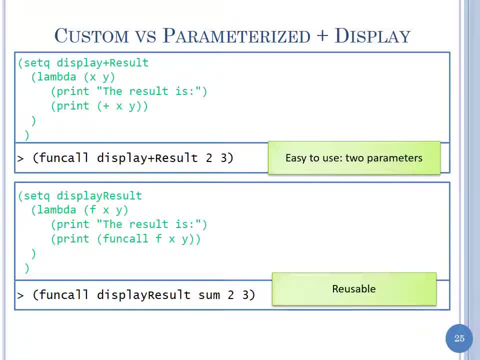 to sort of use it, have the reuse capability and have to have exactly two parameters. So can we combine these two things together: reuse and two parameters? I mean, how can we? This is the question. 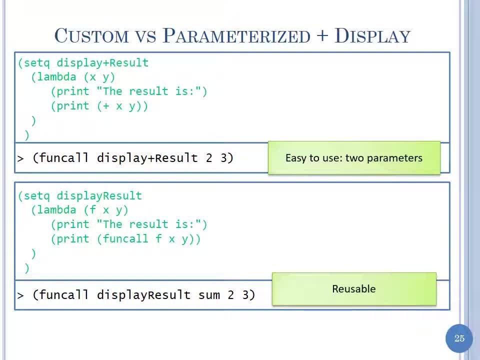 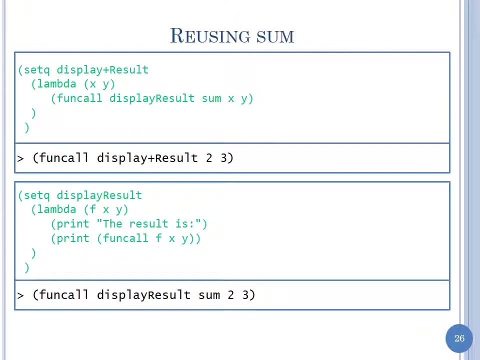 So so these two things don't have to, and I kind of make you go through this process in your assignment three. Yeah, 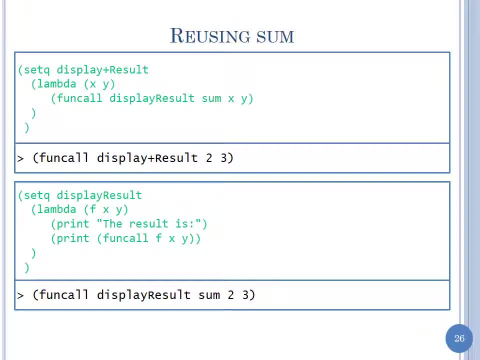 Oh, sorry, I actually. yeah, I wonder I did. I did try to run this stuff, but yeah, I just decided to hardwire everything. Yes, I copied, I copied. this call display results on two, three onto that, you're right. 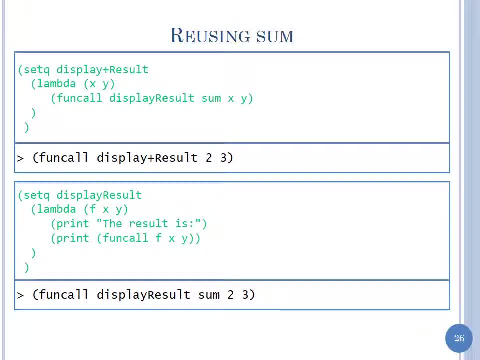 So it was hard to write. These are also assuming you redefined sum. right, I don't redefine sum, I define sum. Plus became sum. Yeah, Oh, okay, Plus was a basic function. sum is my lambda function, Did you? did you type that in as a set to use sum? 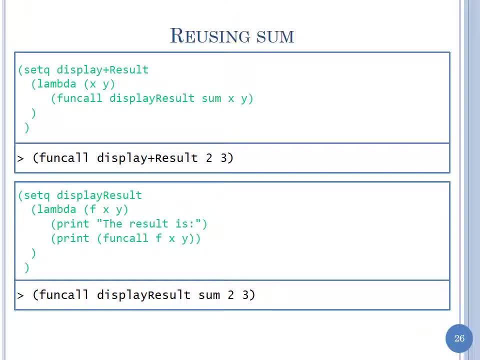 Yes, Lambda, okay, Yeah, yeah, that was way back five, 10 slides away, I don't know, okay, So okay. so, guys, I may or may not correct this, but just be aware there's a typo there. 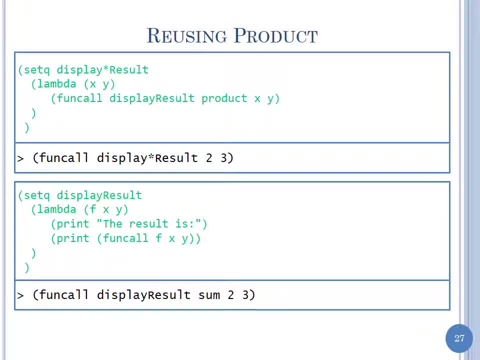 Okay. The joy is, at least I'm not inconsistent. Okay, Okay, okay. So copy and paste is great for PowerPoint at least, Okay, Almost. every time I copy and paste and don't run it, I make a mistake, So that's why I like type languages. 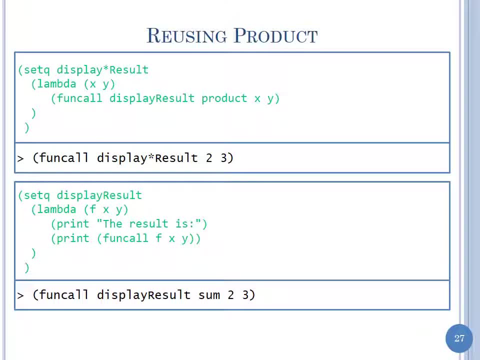 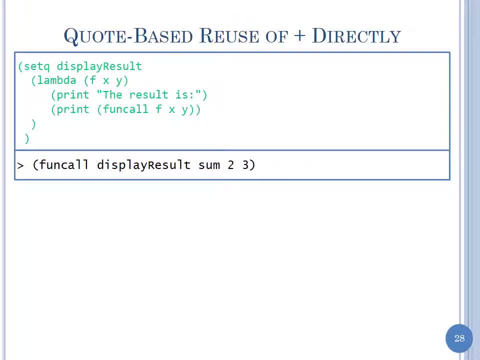 My mind wanders. Okay, Now, when I, when I was talking about this last slide, Okay time, I was very pleased. actually, the three or four of you said: can't we use code plus? and and you know, Ben told us how we could use code plus in C Lisp. so 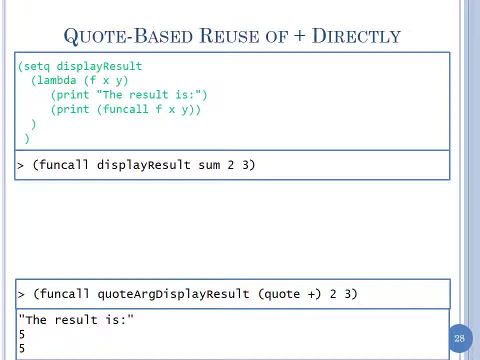 we can't quite do it in our list, but I want to use code plus and I'm going to define a new quote: our display result in case, rather than display result, the display result that takes a code arc. okay, so you see how I'm using it. that. 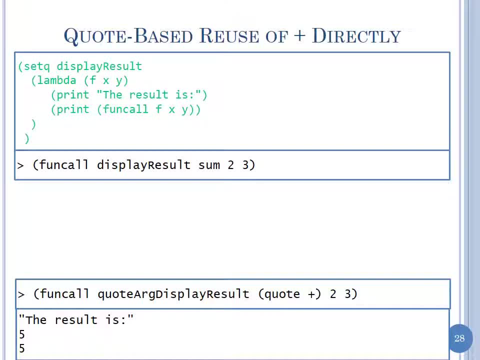 I'm passing code plus and I wonder this result. so the puzzle is: how would you define code R plus? and actually there was a two or three of you who last time gave me the answer, and I don't see at least one of them right now, but but 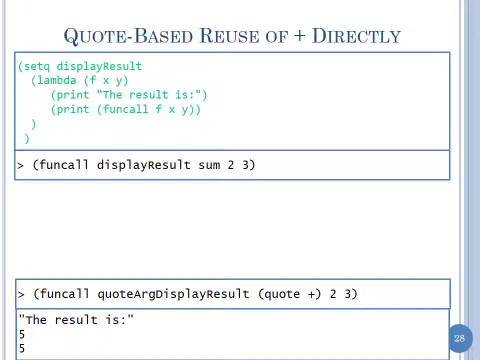 Chris, you gave the answer last time after class, so or anybody else want to say: how would code R plus work? Nathan, you same thing we did in the test. that's what a couple of you said. anything same thing we. so my, you know. I told you that every exam I want you guys to learn. 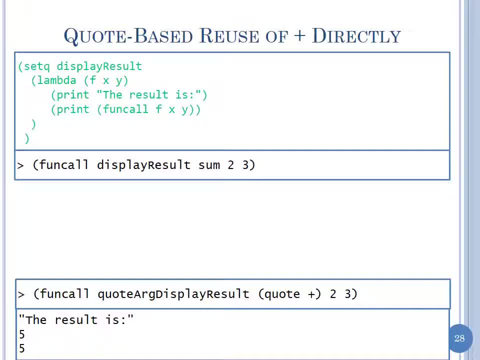 something new. if you learn and apply it to, I mean that's, that's great, so I can. I can do a print list, I can do. I can create a list with that function- okay, and eval that- okay. so this is, this is the kind of way you would generate. you would do it in Java or 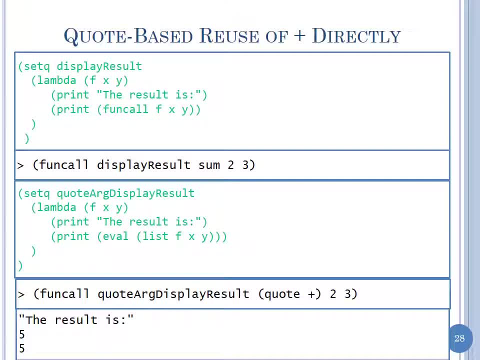 sometimes you just take code and compile it and this is kind of what you're doing. so this is taking using the fact that functions and data structures- you know the homo iconicity of this is- we're really using this here. that function calls our lists and we're just creating a list. that that is then okay. 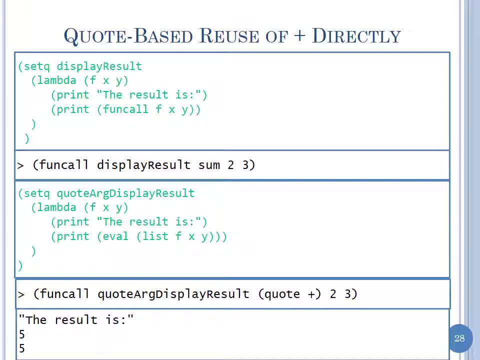 Matt, you have a question. I do the code plus right. so the plus never got evaluated. I then I created a list whose first argument happens to be plus and second, the other two arguments are evaluated to. whatever X&Y evaluated to, then I call eval, if I will evaluate the list and and that would be used as a function call. so 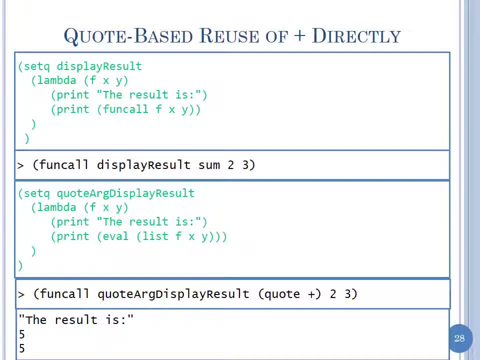 baby, just exactly what we did in the exam. so you want to create a list out of that right. you want to pass to your valid list that consists of these three elements. you need to be able to get to that few of your solutions or to get to that identity structure to find out. 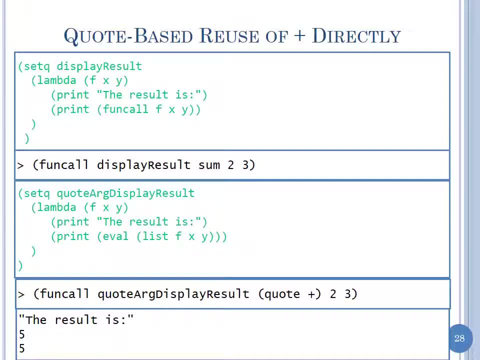 where that identity structure has to be and how it can be evaluated. like what am I saying yes, so that I can take that and I can come up to it, can set up that list. I'll say, yeah, this is the data structure. and then those are the 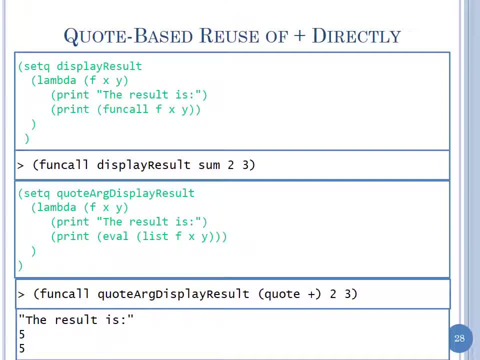 some of the information documents, because I'm somewhere in the different sections in Java that I read you just have two columns on them. I'm desire to kind of pitch them up and set them and promote them to your course or a team. these three elements If we do eval fxy. so what will happen? Let's go and see F will. 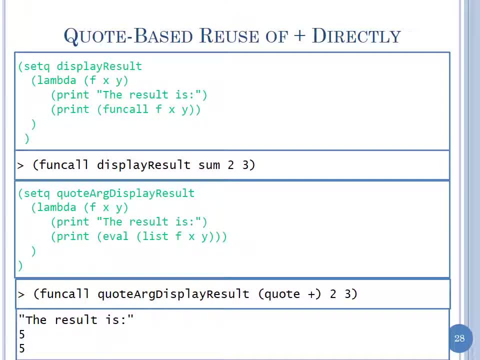 get evaluated to. code x will get evaluated to whatever, okay, And print will get. so print will be, will try to evaluate. so your what print, the evaluator will be called and that's got the tail. so that's a list within a list and you'll have to, I think, your evaluator. 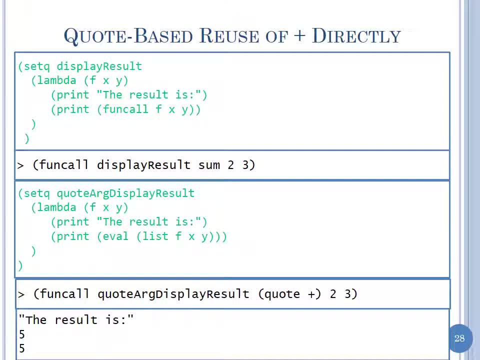 will Okay, Okay, Okay. So the print expects a single argument. it'll get a single argument and it'll eval that. So it depends on what Andrew gives you there. Yeah, but that's different. that's that's so. that's a separate issue. 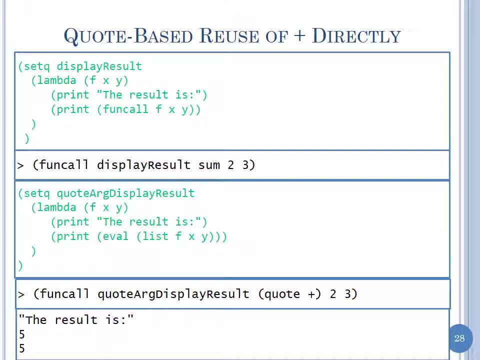 But because in this case, x and y are already evaluated Normally, you you want to say list, because you want to go and evaluate the arguments, okay, So your print evaluator has your tail. so, Yeah, they all consist of, yeah, well, they all consist of parentheses, quote plus and. 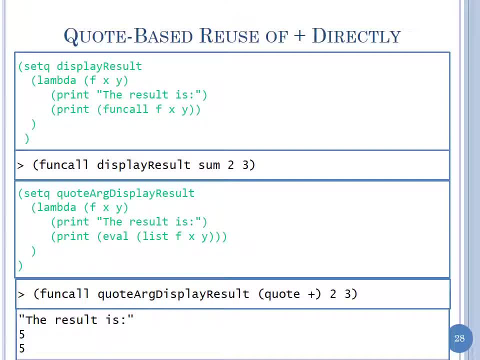 then present is say a term, or x and y, And so then if I you want to go and evaluate, quote, say identifier m plus, And then print evaluates identifier m plus in 3.. No, no, but hang on, hang on. 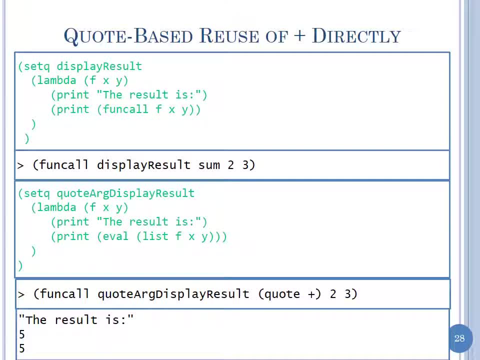 The list that you got was x- y. The one Andrew gave you was have x and y in it. We never got went and replaced that with the x and y that was passed to it. But if it evaluates the plus, it's going to look at its tail and look up x and look. 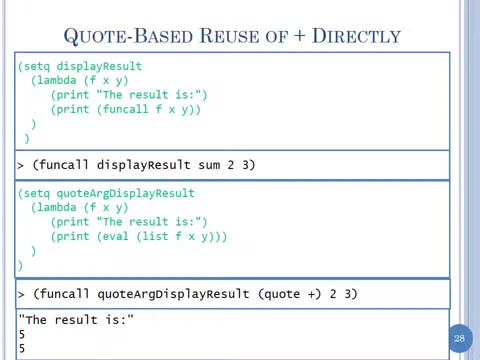 up y. I'm just wondering whether there's an extra, extra list around it, because print will take its argument, evaluate, and there it will. so where did that way did? where did F get replaced by plus? then where did, yeah, where did F get replaced by plus? because print just expects its. 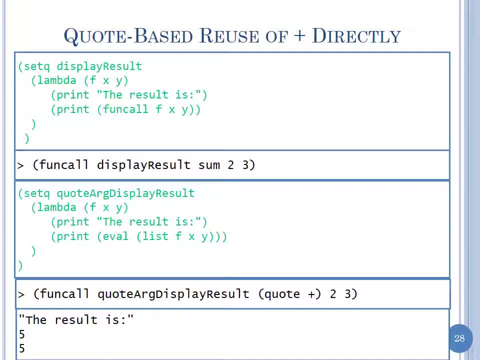 arguments. right, it's got a list, it's got a raw data. this is what Andrew gives you. he's not done anything there. so where did the F get replaced by by plus you? you have to evaluate those elements somehow- X and Y, you know? if we could? 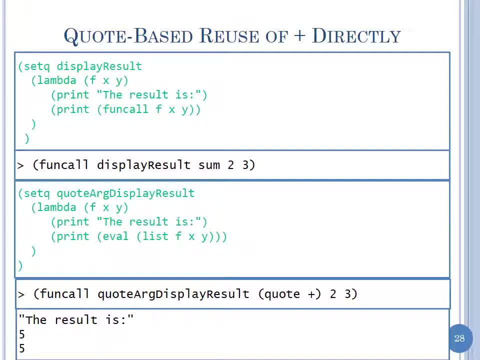 somehow make that become plus, then X and Y will get evaluated. but print never got. F never got replaced. so it will look up the evaluator for F and not plus. but by the interesting thing is you can just run it in interpreter and see what happens. but that's. I think that's the right answer. 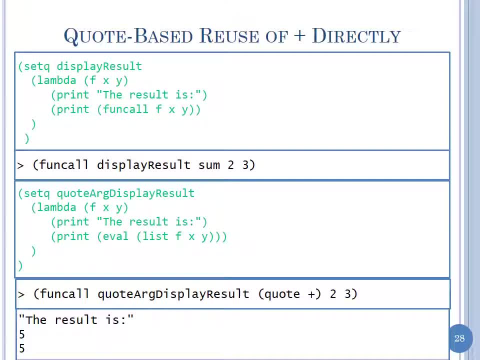 okay, questions. so do you guys get that? instead of saying list FX, why, if you just put FX why there, what would happen? okay, and that that would be a sub list that and was created. you cannot evaluate that that sub list will. then you know, go and use the look up the first argument, go and see whether it is something you 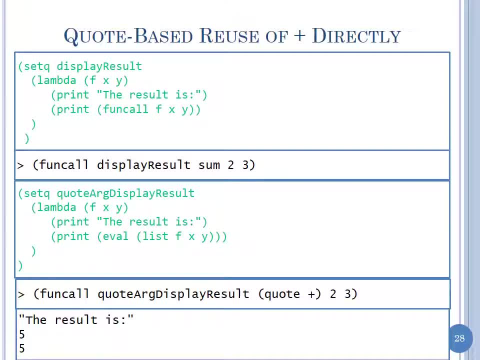 can look up. f doesn't have to happen to have a value, so it'll go in. it'll go and just give you that error. so you somehow want F to be evaluated and X and Y have already been evaluated. and if it was calling that particular plus, then X and 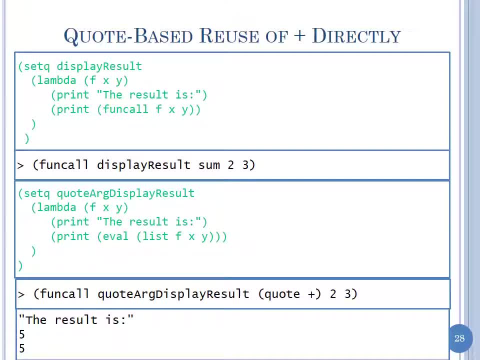 Y indeed, would get and looked up okay Questions. See, this is why you need form formality. okay, to answer questions like this, either you need to sort of prove something or you need to go and have an implementation. in fact, implementation is so. it's not a mathematical, but it's a precise definition of something. 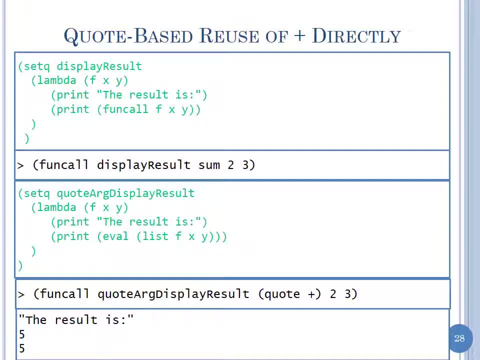 yeah, so you're saying f is already bound in the current environment and when you go and do f, extends have to be fun, call right because f happens to be, oh sorry, f has to be plus, so f is. if you're saying f is in in your environment, 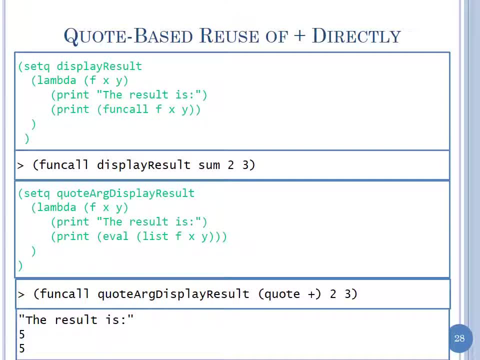 so. but but we don't expect pluses to be in the environment, right? we expect plus to be a basic function. plus has got no lambda expression associated with it. we want the evaluator plus to be called used, no, so. so the thing is this: when we go and call a function, f cannot be. when we just say f, x, some. 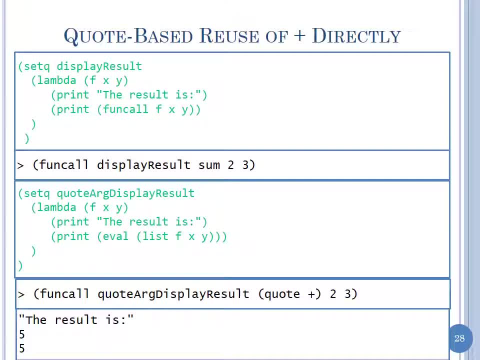 function called f, x, y, f is never evaluated. fun call f is evaluated. if you say fun call f, then that f is evaluated. if you just say f, x, y, f is never evaluated. you go and look for an evaluator for it. f is in your environment, but it is not in your evaluator registry. 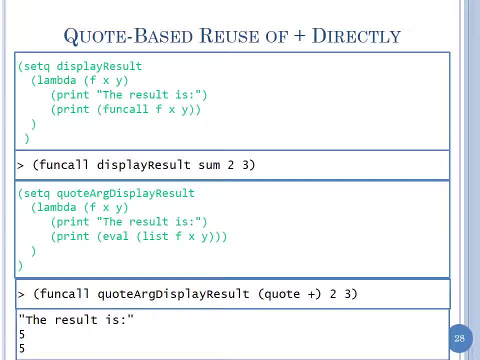 but i'm dying to sort of go and see what happens in the code. okay, but i suspect that's what's. that's what's going to happen, because you're so. just remember, right now we have two ways to call functions. okay, we can say: fun call. 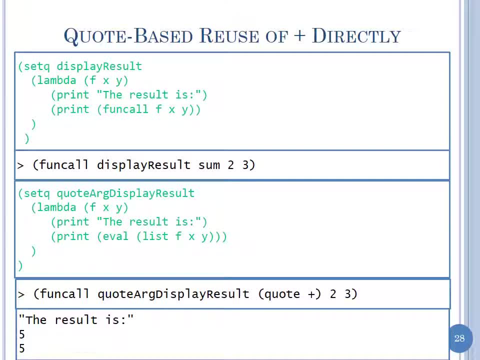 f where f is bound to a lambda expression, or we can just say f without fun call. we haven't done different defense so far in our interpreter. if we just do f, it looks up in the environment for a lambda expression. sorry, if you do fun call f, it looks up the lambda expression. we just do f. 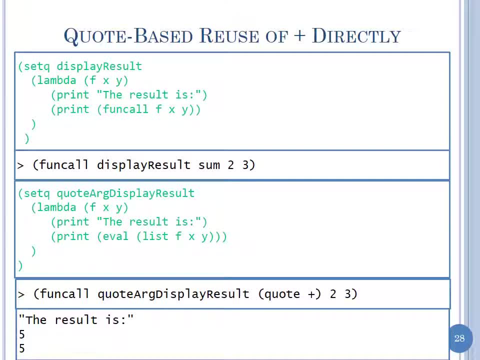 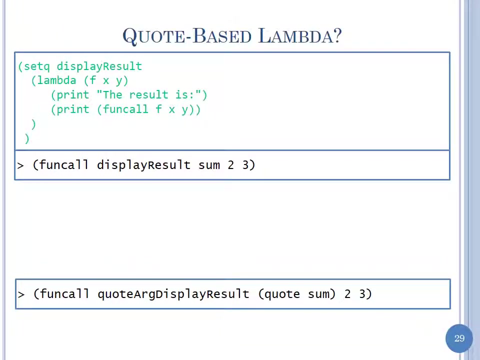 it looks for an evaluator named f and there is no evaluative of f. okay, okay, but is this good? okay, so could i do this? now that i have that code, can i say: uh, code sum, because this is not a fun call. okay, so, uh, undefined function sum. okay, it looks for. it looks for an evaluator. 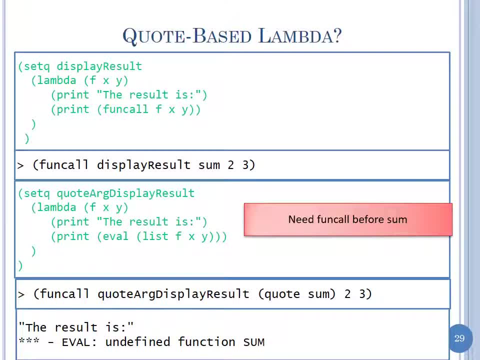 it's with sum and it doesn't get okay. so we have to remember that basic function and lambda expressions are two different things. okay, and when we define, when we do define, it'll kind of mix them together. but the fun also expects lambda expressions. sorry, first, yeah, so in our, in our interpreter, we can't say: fun, call plus. 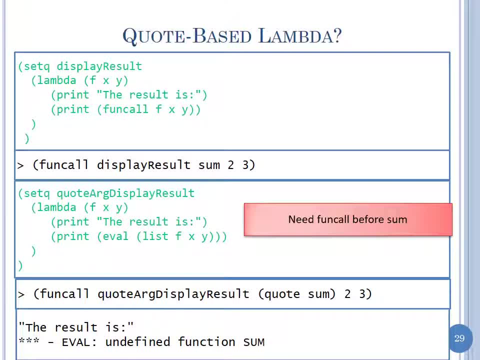 in ben's interpreter you can, in c list you can, but in our interpreter you can't. say: fun call plus okay, we always expect that to be lambda expression. that's more uniform. it's not very practical. you can do special casing and say: oh, if that happens to a basic function, i'll do the basic function. 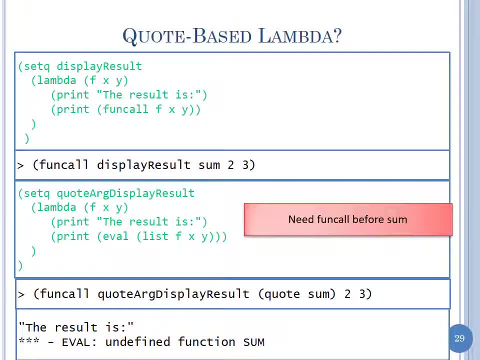 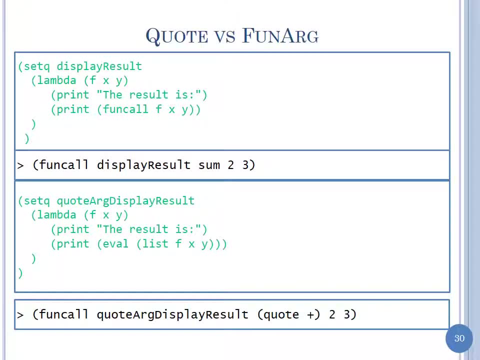 thing. okay, so, so, so, so, No, no, no. Okay, so we've seen that we can reuse coding two different ways. Okay, we can have fun. you can have something that is a lambda expression or something that's quoted, so we can do a fun call. it should really be. 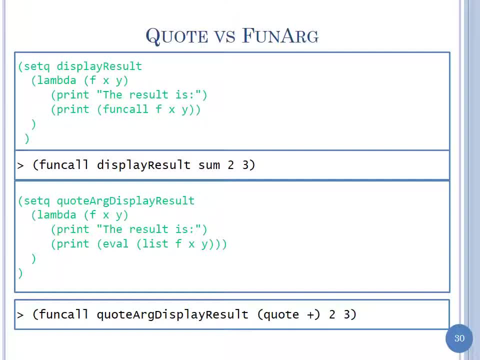 uh, two ways of doing things. forget the fact that plus assume that we've got a C list like or bend like thing. which do you think is better way to code? so forget the fact that you can't. you know, sum and plus are kind of not interchangeable right now. for now, just conceptually, from from understanding the 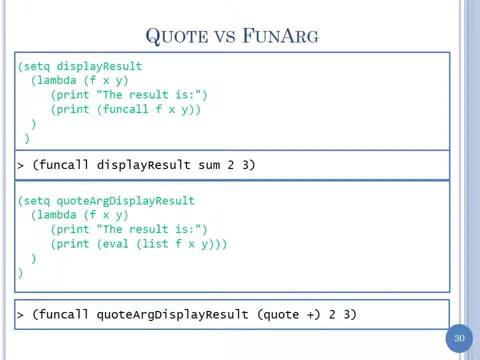 code which, which, which to which? to you, you is more understandable, Chris, which one? the the, the first one, the second one? why? and you're doing fun call, it tells you you're doing a fun call, okay, whereas here you're building up a list and you're evaluating it and you 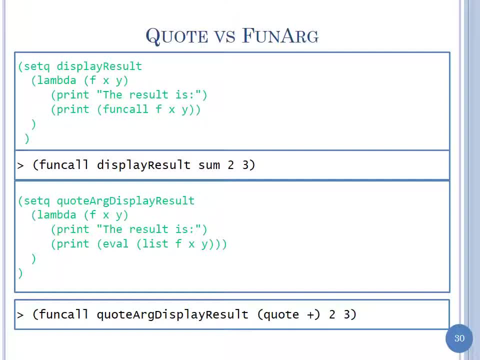 know and think about it, that supposing you had a programming environment that actually gave you help with filling in the syntax by telling it you're doing a phone call, it can go and make sure that you're doing certain things. if you just say that list, it doesn't know what kind that list is supposed to be. it happens. 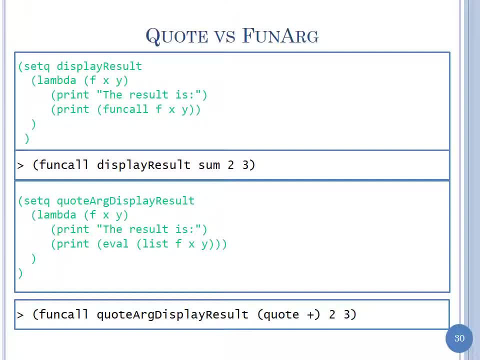 to be a phone call there, so probably that first one. okay, can we do the third way, whether we like it or not? I mean, you know it's good to go and understand all the obscure ways, like I said, also because you might, somebody might use an obscure way. can we somehow do reuse with with function returns? 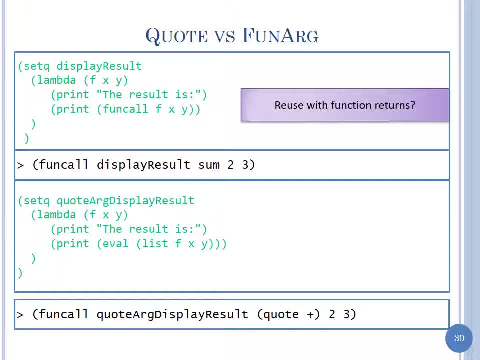 somewhere? here too, can we bring in function result: it returns and actually the reuse is occurring. yeah, let's, let's go and just see how. can function return somehow play a role here? yeah, I don't know either. I haven't provided the full motivation I want to. 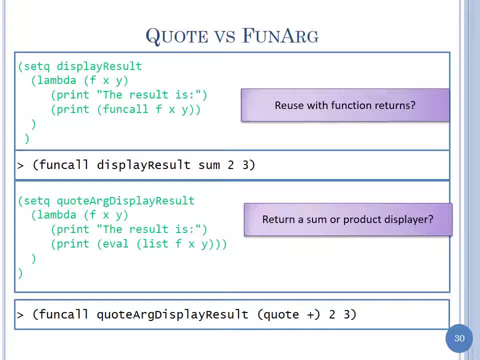 use function return somewhere in this problem. okay, I want reuse there, so let me- actually I don't have the right slide, but remember how we and how we define display, this plus result and in terms of the fan art display result. remember that where I made a mistake of 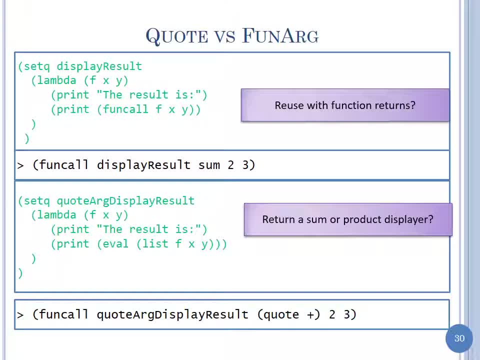 two, three and XY. I don't want to do that. I want to have an alternative to not these two things, but an alternative to the display plus result that involves a function return somehow, so that function display plus result called my display result. right, it went and called in this body. 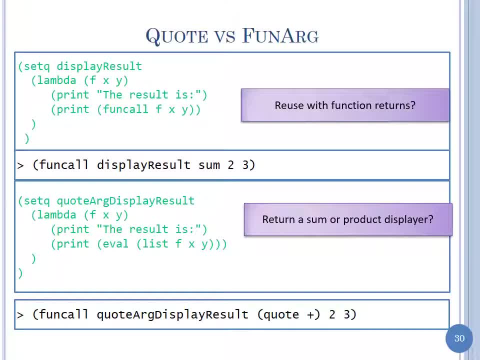 and I want to go and somehow generate that function display plus- as a function return. and you know, I might just have to sort of give you this answer because I tried to make everything. I say something derived from a question, but you know, making the slide I wasn't sure, but anybody want to think about somehow? yeah, 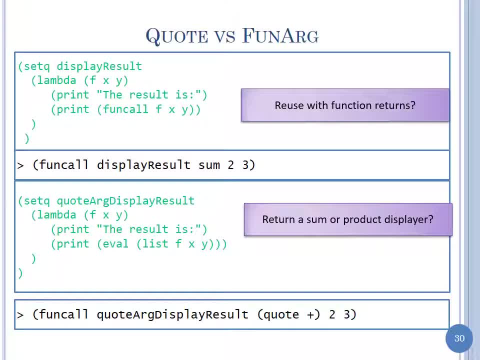 no, I want to somehow get function return here. I want to build something that will return a function that I can then call to do the sum. that's my thing and I want it to be reusing so. but I want to generate a function that I then go and call to get the sum. that's what I want. 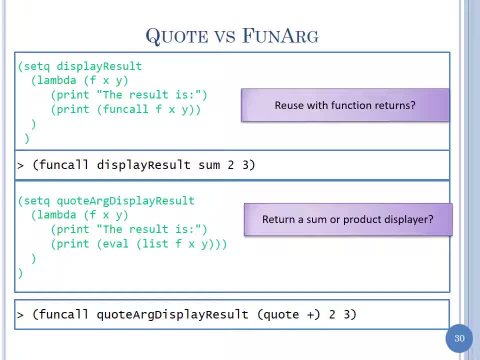 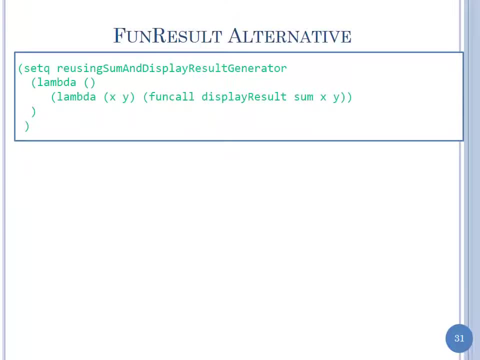 to do you A little simpler than that. I have a generator and we're going to play with this little later when we do currying, to make this more what you motivated. but this is something we can do right now, which we can't- the currying stuff we can't do. 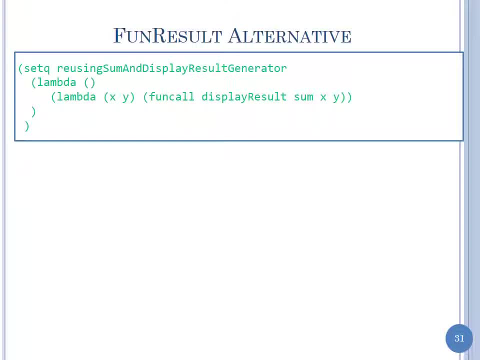 right now. I have generated a function- not the more like a function, that's like like a- but we have generated a function that is like a null function. but we have generated a function and we're going to create a sum function, display some function. this function takes how many parameters the 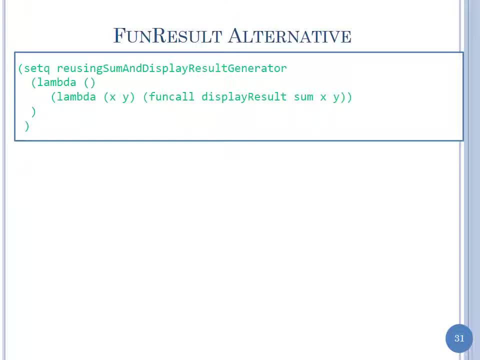 function that I'm just showing you we are nesting, like Nathan was suggesting, I'm returning. I'm returning a function takes how many parameters zero. the function of returning returns. it takes how many parameters two. so the function i'm generating does what it does. the display result: uh sum x, y. so i've generated a summer display- summer rather than. 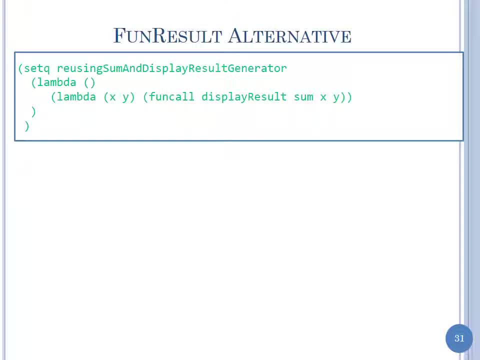 just going and hardwiring that and later we'll see that we can actually pass a parameter to this doctor function to make this more modular. so i can go and say func call. so there are two levels of fun calls. i first do a fun call to get the function. 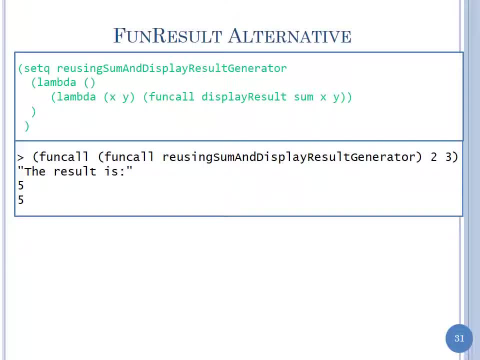 and once i've got the function, i go and then call the return function with arguments assuming: yeah, yeah, yeah, so this is this is. you know, this is not that motivated right now, okay, and we motivated later. there's a guy called haskell curry, after whom the language haskell was invented. okay, named and off. 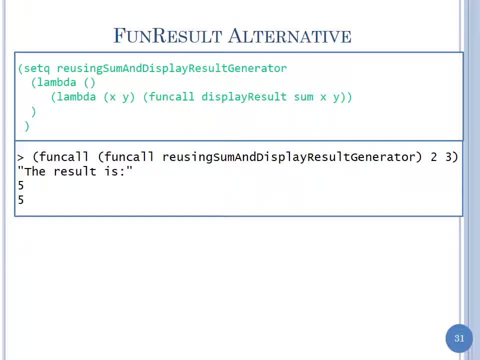 and the curry was used to use. he'd love to return functions and, and and we'll go and look at the curry operator later later to sort of make this more useful, but um, but you see at least what i'm doing. i have a lambda, i have a function that returns a function. 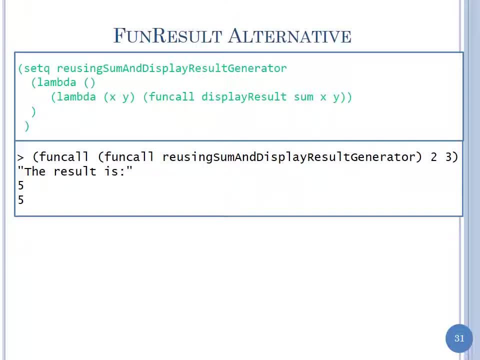 so- and i do this kind of stuff in java too, by the way, believe it or not- i, i take java. i take a piece of code, i generate a piece of code based on my current state, i compile it and i run it okay, so it's a little. 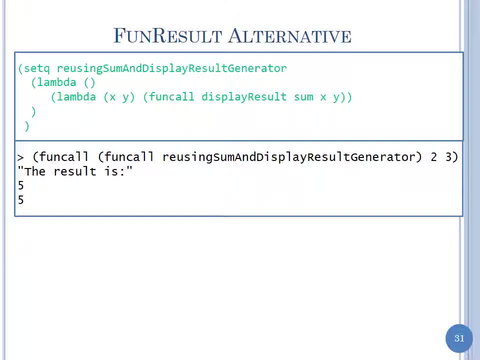 bit more awkward in java, but this facility is: you know, you have a lot of generators in this world and and so you know that's so. that's the function. so again, let's make it very clear what's happening. i have a function that just takes no parameters. 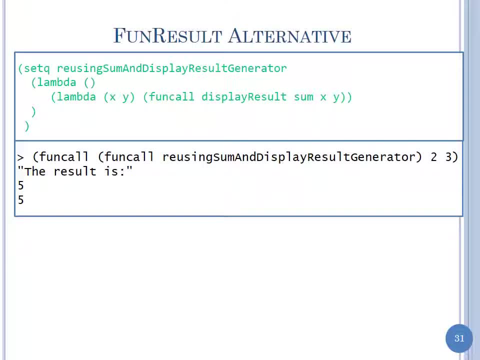 and it. it goes and returns a lambda expression, not an application of a lambda expression. what we saw in the previous funk displayed plus result, it was that there was a lambda expression that went and applied a function in it, in its body. here we just returned the lambda expression which takes two parameters. we don't apply it, okay. again, i'm trying to show you. 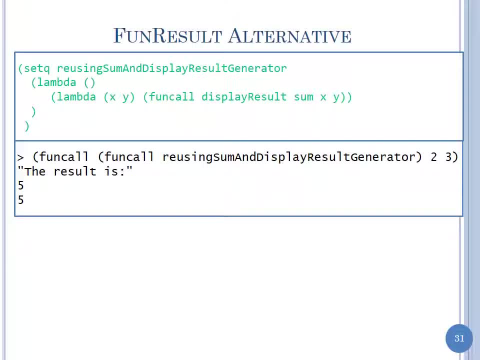 how we can use anonymous lambda expressions. and then the idea is that once a lambda expression is returned, i'll go and pass it parameters. so i do the inner func call to first get the function- and that's why i'm calling it a generator- and then i'm doing the outer fun call to. 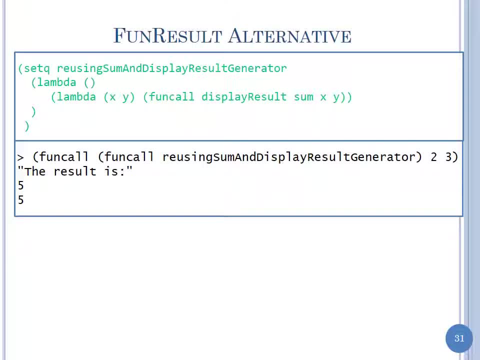 apply these arguments to the lambda expression that was returned. okay. and this will all become much more concrete if, right after this class or today, you go and do assignment three. okay, this is the time to do assignment three, first part. everything is fresh in your head. consolidate that and and and. uh, you know you learn some of the 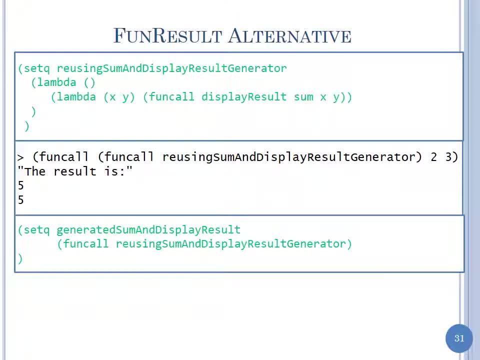 deepest things in functional programming. okay, and what i could then do is i could also do something like this: that i i i take the return function, assign it to a variable function. okay, so that i don't have to go and do this nested fun call each time. 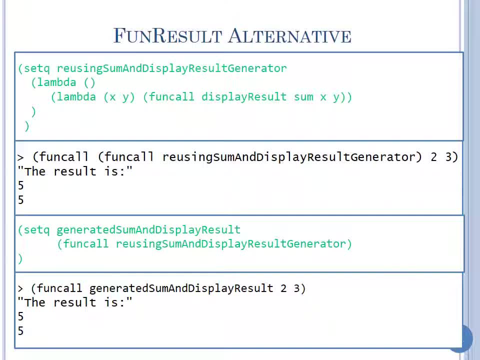 and i can. i can then just keep applying this return value again and again. this is what this was invented for in: to actually generate programs at runtime that learn things. okay, it was not all this machine learning thing, but it's all done through statistics. the idea was you. 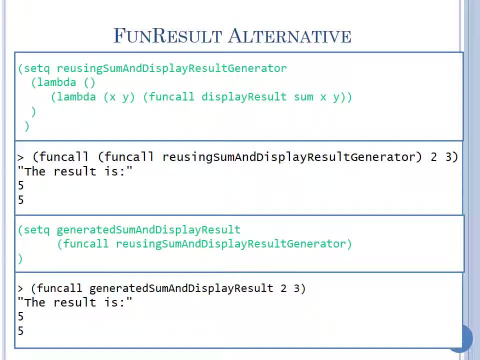 were generating code at runtime by learning things. okay. so you actually generated this particular function and you've gone and then stored it in a variable- okay, homo, iconicity. and then just do a fun call on that and you've got this. okay. so this is all all that you need to do. do this first part of. 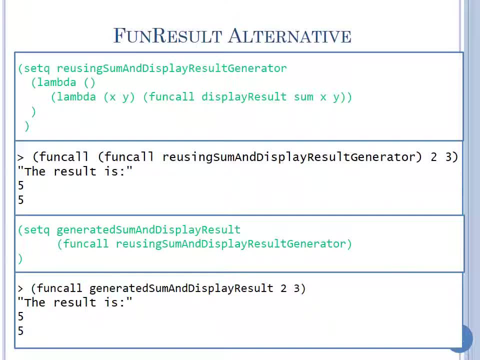 the assignment. yeah, um, func call that the func call it's. it returns a lambda it takes. we don't give it any arguments, right? so that func call returns a lambda expression, which I am then passing to the outer. func call the inner. func call returns a lambda expression, the inner, remember the, the, so what? 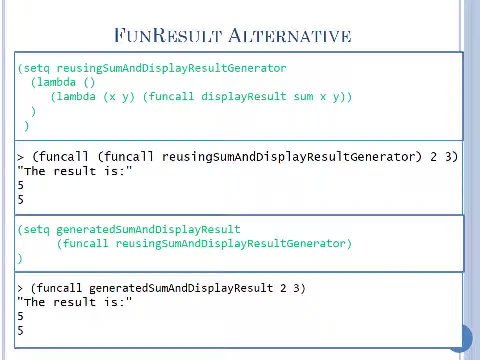 was outer. the outer lambda is the inner func call. that's the confusing part: the outer lambda and then in the in the definition becomes the inner func call and the inner lambda and the definition becomes the outer thing, because we are returning things. so this func call, this func call, returns this lambda expression and to this lambda expression, this lambda, 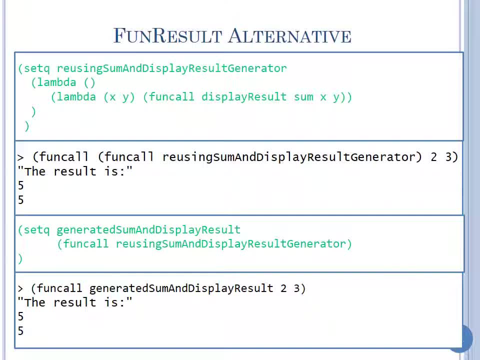 expression takes x and y, to which I am passing 2 and 3.. And I am doing this in gentler steps. here I am saying generated sum and display result is assigned to it: func, all this. So I get this lambda expression stored here and then I say: func all generated 2, 3, which is just saying this in two different 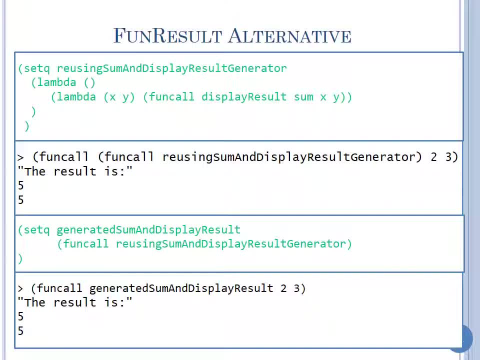 steps. That is what you expect from return functions. right, you return a function and then the return function can be applied. So one func call to return the function, one func call to go and call the return function. yeah, So I have this sort of like a question. that is something I had before. where we are, 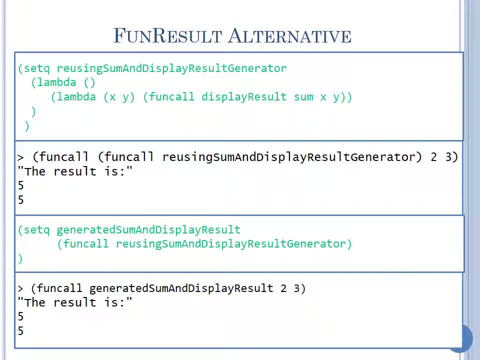 but I am sort of curious if there are any other functions like that. We are using set new line, why? I know that we don't- Yeah, We don't know how much defun really works yet, but why do people use set new or defun? 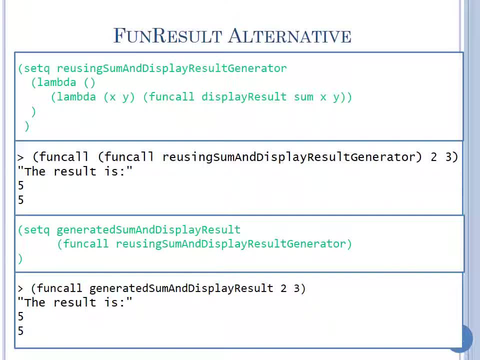 Is one of them inherently better, or like because if you are building an encoding style and you use a lot of set new, so you can func some more, Okay, So what are defuns and why are defuns? and I didn't even know about defuns when I 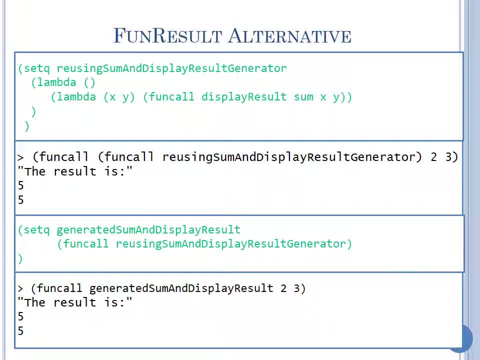 was studying this, okay, So I have very carefully tried to layer list, you know, since I believe in layering and you will see how carefully everything is done. So defun will use set new and will be conceptually use set new and some other concept we are going to look at. 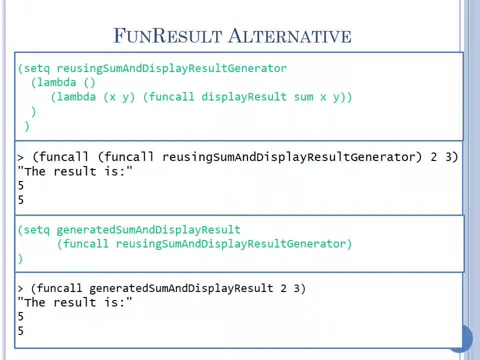 and then it creates a different namespace. So it does two or three things differently, but we are gently going towards it. but we don't need defun right now. okay, We have got. we need something else, which will come to next. There is one more thing we need before. 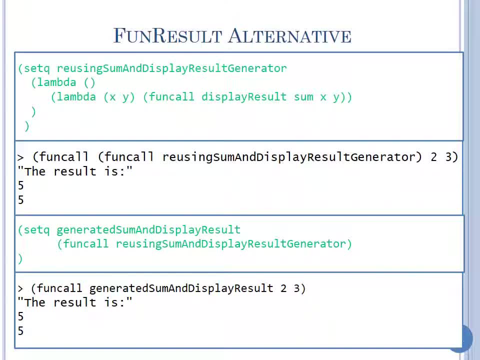 we can really really use return functions. So there is a reason I can't do currying right now, Because there is one very important thing that there was discussion at Piazza on about which we haven't done. No, no, no, that set. I hate set queues, So, as you should, I mean. 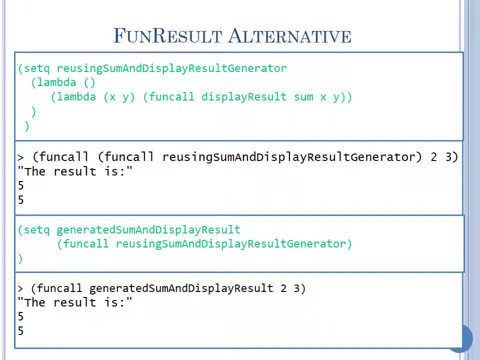 you want to have as few set queues as possible and you want to have set queues only of functions in the good old lisp- okay, the functional lisp. So later with curry operator. fun result will be better motivated. but this is what we seeing here is fun result. So at least. 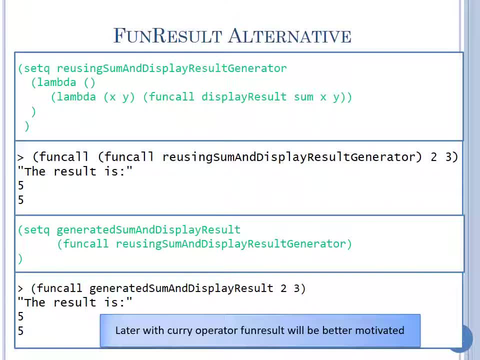 you guys. and, by the way, if you do C programming, you can return. you can return addresses in C right In C programming. you will see lot of stuff like this, okay, So it is very important to sort of understand, understand this concept. 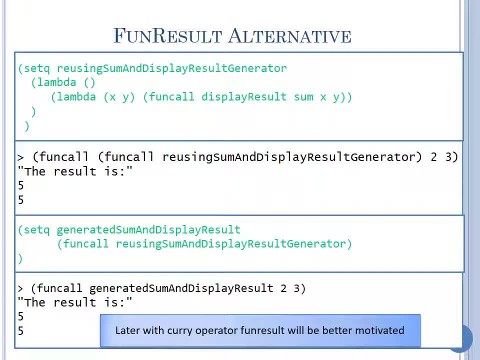 But what type safety do you have here, Except that you will get an error rather than go down right? So, yes, having program in C and lisp both. lisp was more friendly, but lisp also is, as you have seen, your, you know, you know you. better not make a mistake in lisp. 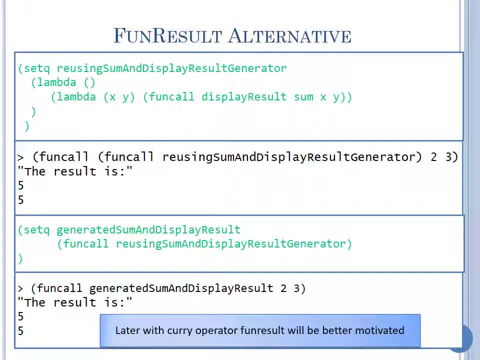 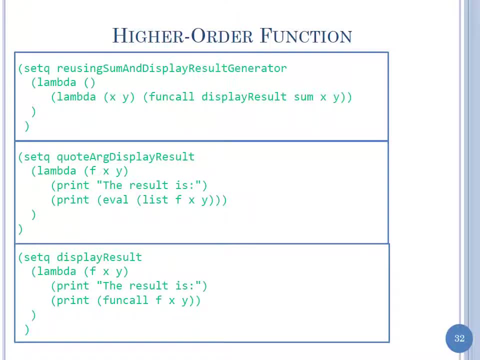 either. okay, Okay, questions. So the term higher order function is often used, and can somebody want to define what a higher order function might be? Well, I mean, you know that here is a term, here is something we have learnt. try to fit the term to something. 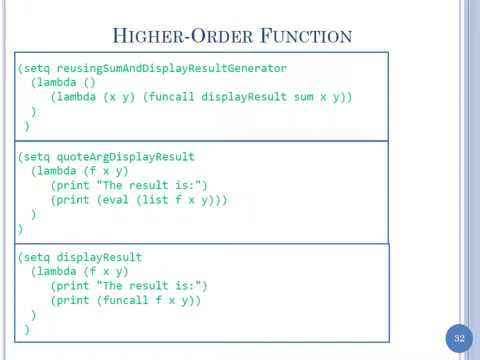 we have learnt: Function that returns a function. Function that returns a function, that could be one definition and somebody want to have an alternate definition. If it uses a function, then you know if I, if, if push, push stack uses array dot lists. 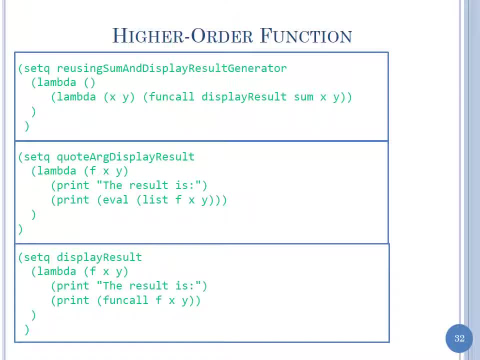 that is not quite the same thing. Uses a function. if expand on that, it has a function argument. Okay, and if you actually go, the argument thing you can get: a first order function is function that takes, no function argument. second order function is a function that takes. 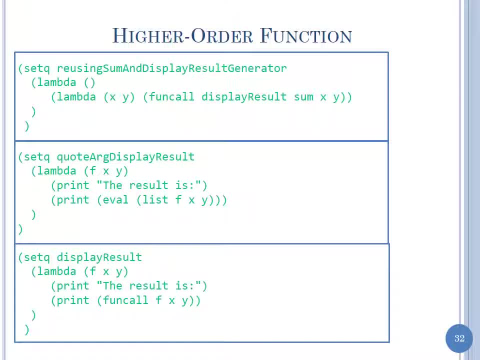 a first order function as an argument. nth order function is a one that takes n minus 1 function argument. okay, So function whose arg or return value is a function, and it could be a name, it could be an address, in, in, in C, or it could be lambda expression, that is. 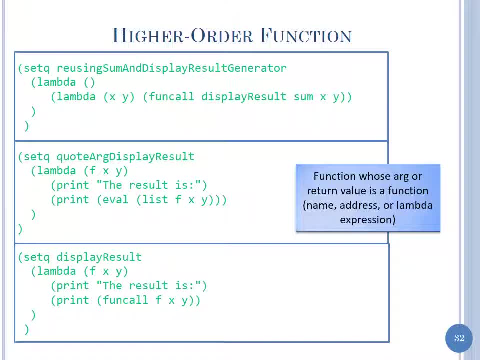 a secondary thing, but it is basically a function That manipulates functions. essentially Okay, and real functional programming involves higher order functions. Is it like? I know vector is used in classes, but is it sort of like that public function that? 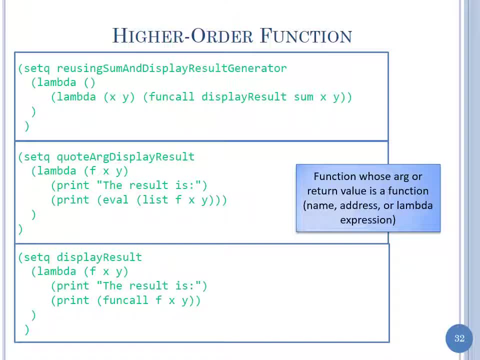 Yeah, it is like a class class using another class. yeah, yeah, yeah, Okay. so let us go come to kind of Nathan's question: What are we missing? I mean, forget this. define, define. lets you go and not have fun call and and and with 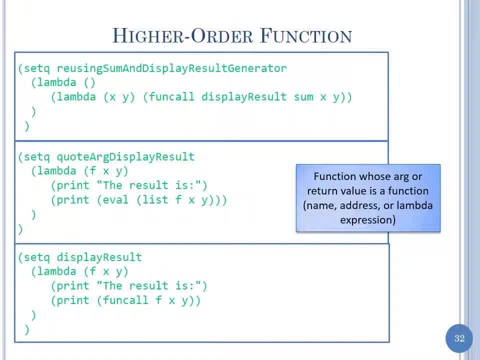 fun call. we know that we can take the f and it be evaluated, which is very nice feature. What do you think is really missing so far in what we have done? Something fundamental, something conceptual, And there was a Piazza discussion on this aspect, actually. 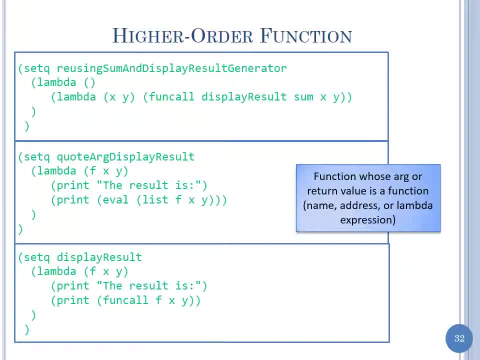 Nathan. Yeah, let us not change global variables. I hate them. okay, Let us let us look at functional programming. Yeah, scopes, scopes- you can have more scopes. okay, So there is something called let that allows you to have more scopes than just two scope. 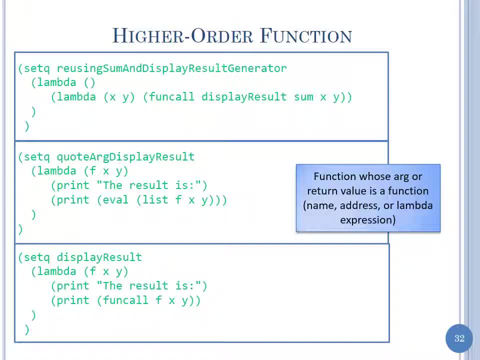 just more statics. Yeah, I am kind of giving the answer away here. So there was a discussion, there was a question asked at Piazza and Ben and Tao is Tao here. They got into a discussion on, they gave an answer and I do not know who Tao is, but there. 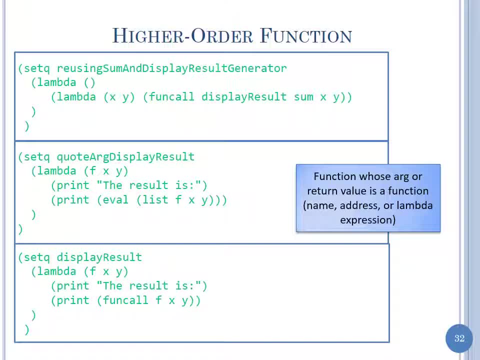 was a guy called Tao Tao who also was involved in the discussion, and it has to do with scoping. So there is, when you return functions, the question is, what is the scope of the function? okay, And there was a discussion and people talked about lexical scope. 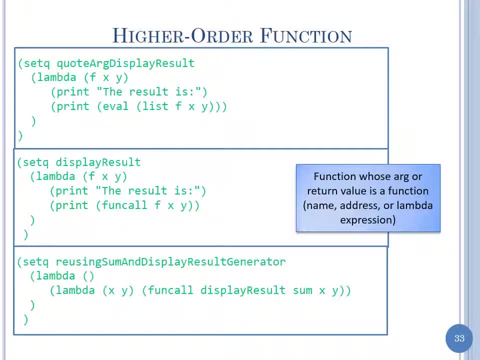 Okay, so what assignment three, part one, is about, and what we considered in the last couple of lectures, I guess, is higher order functions, And we said: a higher order function is a function whose argument or result is another function. okay, 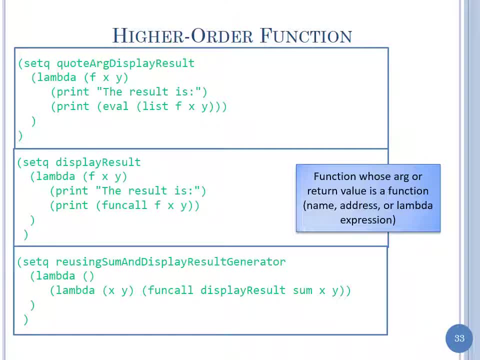 And we saw three kinds of higher order functions, two of them that take function parameters and one that returns a function. And we saw we could write a FunArc function either using a direct function parameter- I mean, which could- which either does a fun call or does an eval. 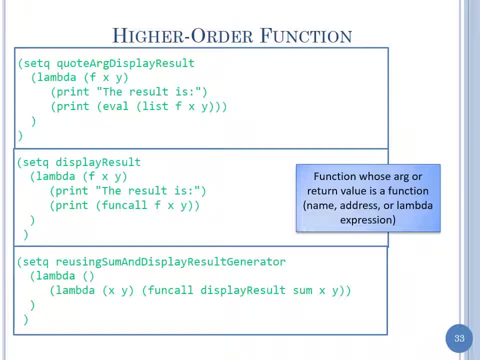 And when you do an eval you can just go and pass directly basic functions And when you do a fun call you have to pass lambda expressions. Okay, so the first one does an eval, So you say print eval, you create a list that describes the function call and you